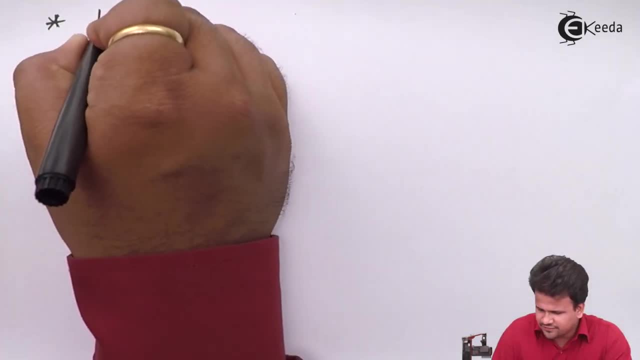 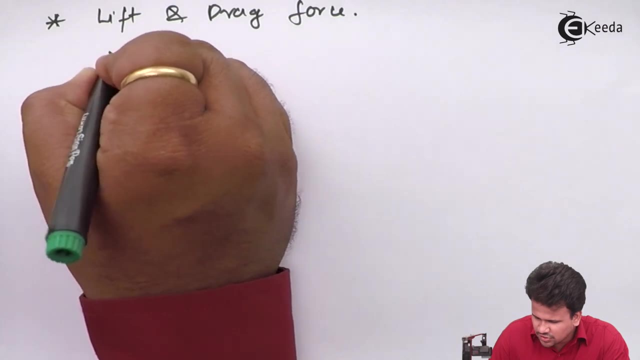 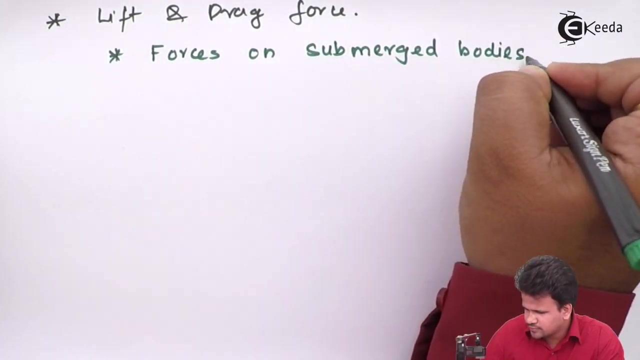 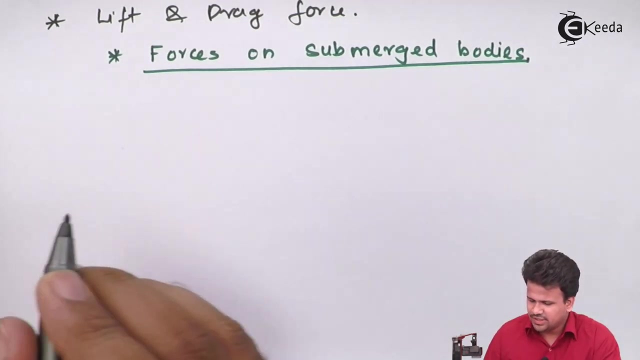 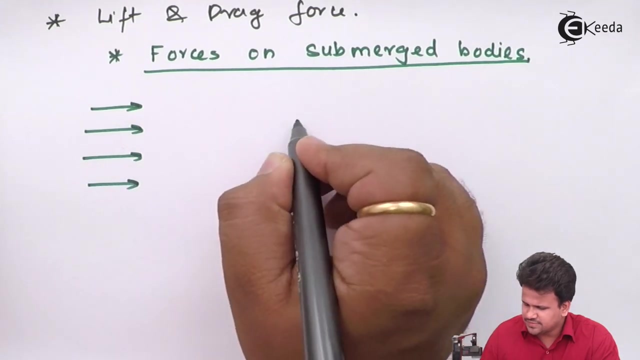 Now, before learning what is lift force and drag force, What is actually? forces on submerged body? Now, what are the forces on a submerged body? Now, let us understand this. Now, if a body is there- supposing this is a random body- and air is flowing at some velocity, u 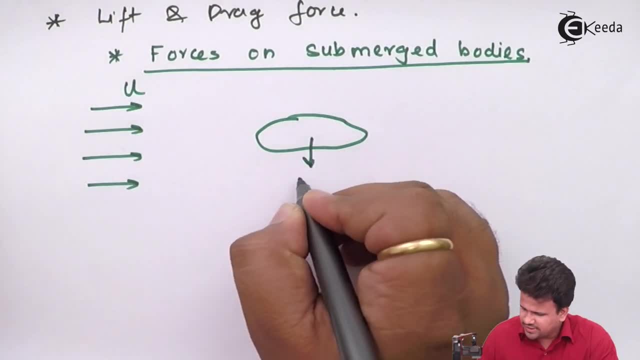 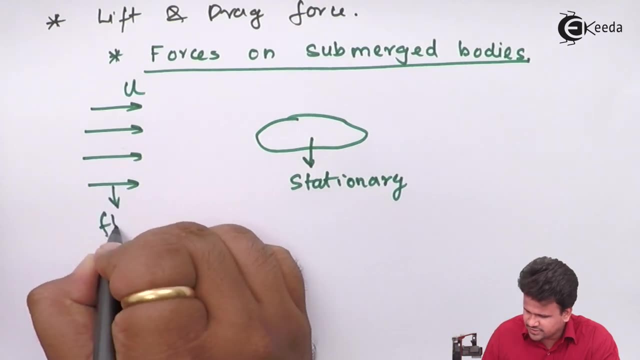 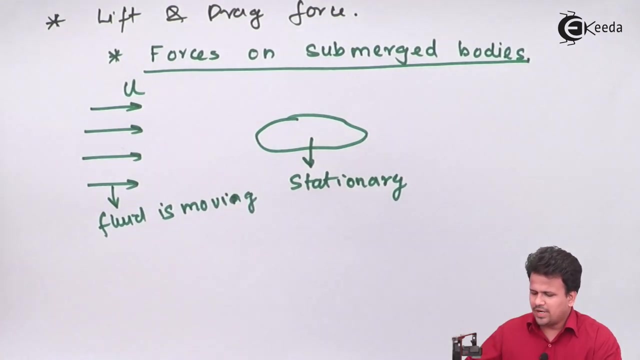 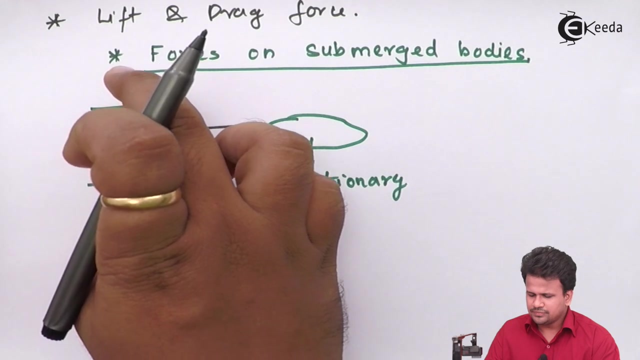 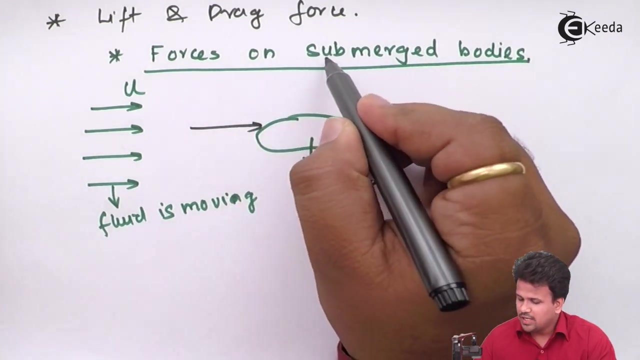 So this means the body is stationary And the fluid is moving. Now, during this, what happens is there is some force which is induced on the body by the air. Now this happens when body is submerged in a fluid. Now there are two cases of body submerged in a fluid. 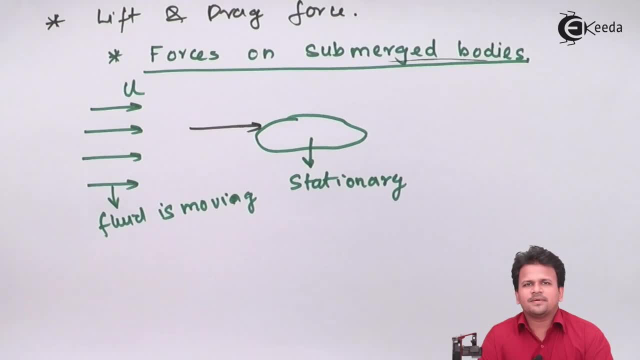 If we take an example of a submarine which is submerged inside water, So that we can consider a case of body which is submerged inside a fluid. The second condition we can consider is the atmosphere. So we live inside the atmosphere. So atmosphere consists of air, which is also a fluid. 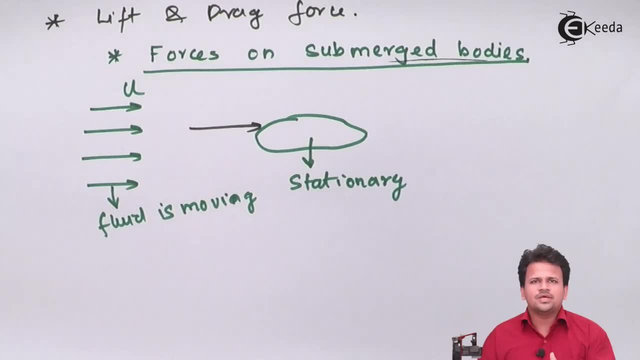 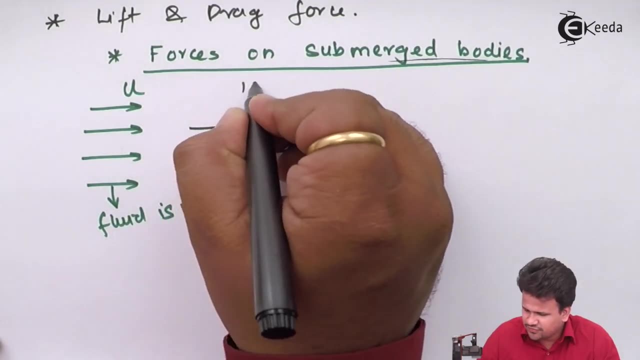 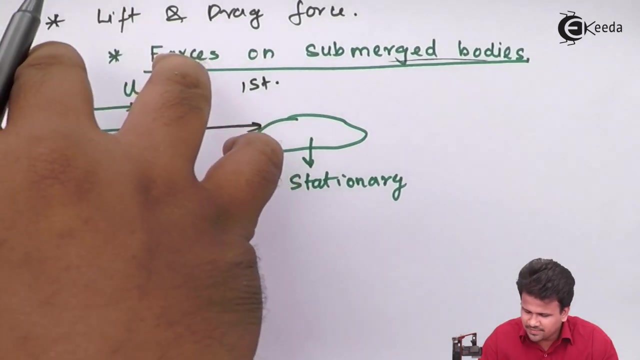 Now we are also submerged in a fluid, which is air. So now there are two conditions we have to understand. The first condition we have already considered, that is, the fluid is moving and the body is stationary. So there will be some amount of force by the fluid on the body. 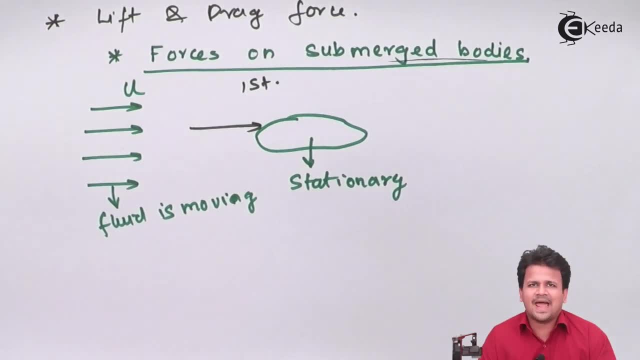 So that force will be called as the forces acting on the body, Now that forces will be responsible for drag as well as lift. Before learning this drag and lift force, let us consider the second condition. The second condition will be a condition where the air will be stationary but the body will be moving with some velocity. u 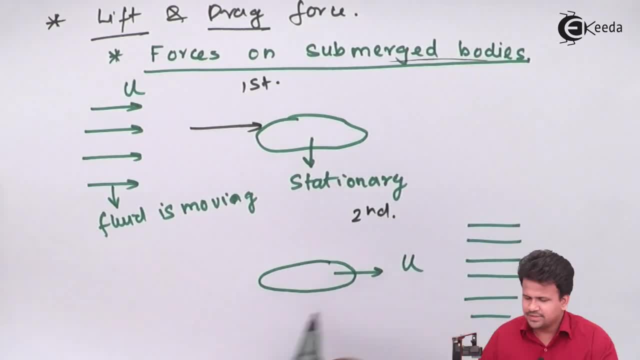 So air is actually stationary and the body is moving with velocity u. Now, during this, since the air is stationary and the body is moving with some velocity u, There will be some induced force by the air on the body Because it is cutting through the various layers of air. 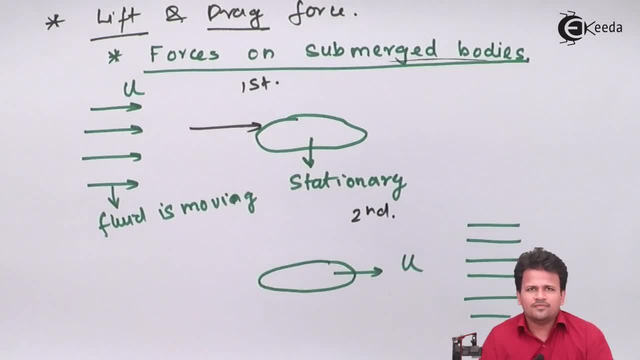 It is same as swimming through water. So if we have to swim from one part to another part, we have to apply some amount of force, Because it will have some amount of viscosity, and we have to overcome that much amount of viscosity of the fluid. 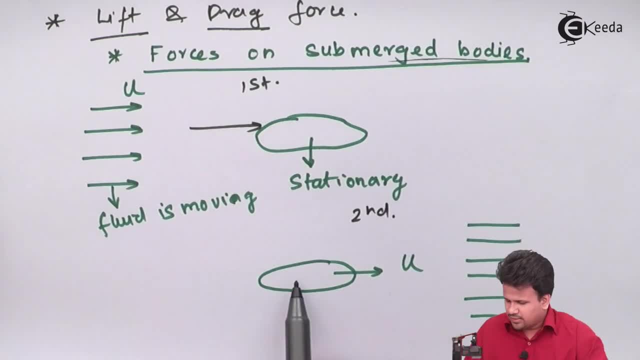 Similarly over here also. if we are going from one part to another part, we have to invest some energy. That investment of energy will take us from one part to another part, But during which there will be some amount of friction. The friction may be a solid friction between the two rubbing surfaces. 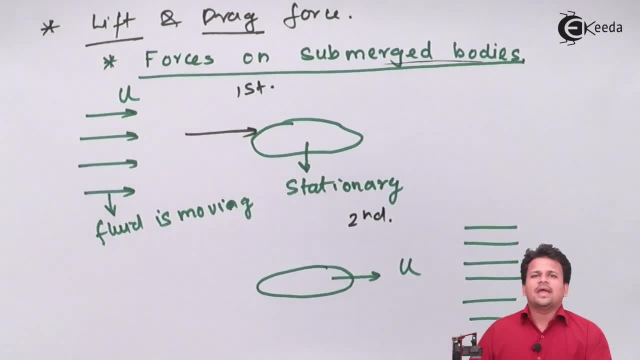 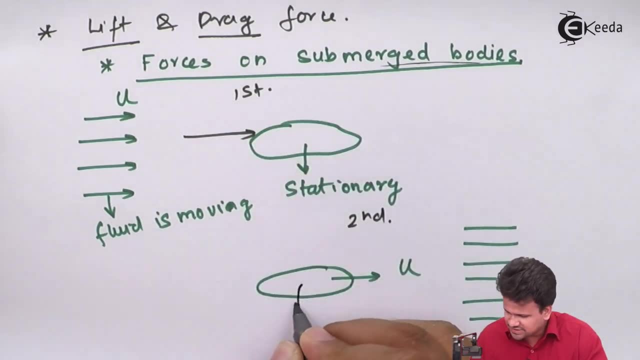 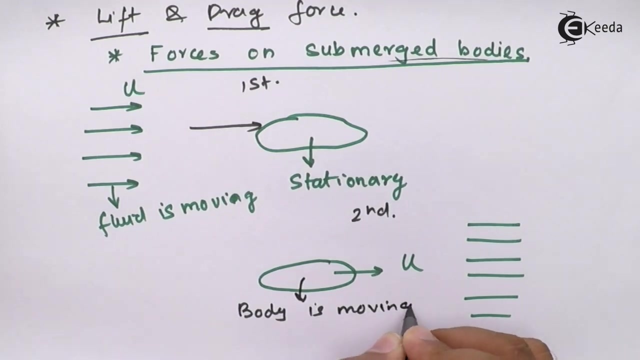 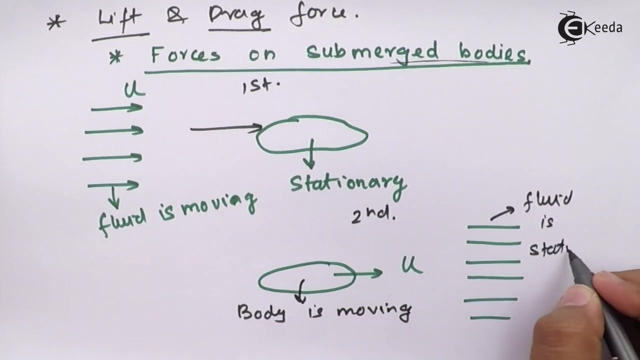 And this is called as the fluid friction, which will be induced by the fluid on the body. So these are the two conditions. So the second condition we can classify as body is moving And the fluid is stationary- The effect of force. 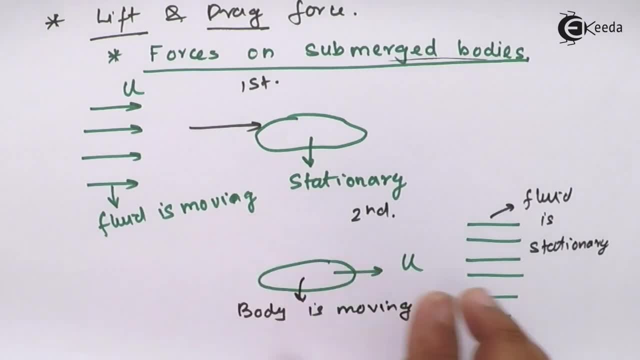 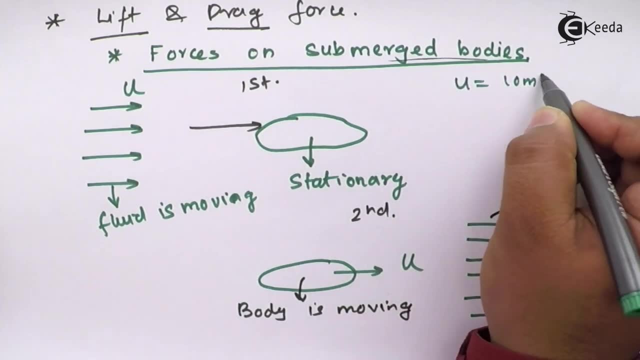 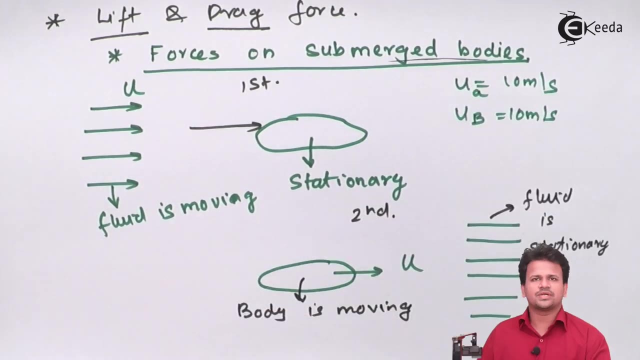 The effect of force when the fluid is moving or the body is moving at the same velocity. If the, for example, the velocity is 10 meters per second, If the velocity of the body is also 10 meters per second And the velocity of air is also 10 meters per second. 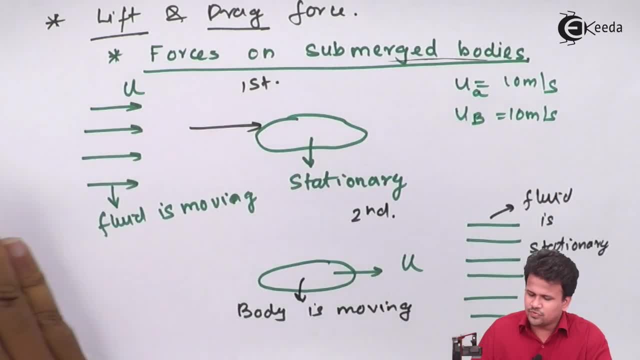 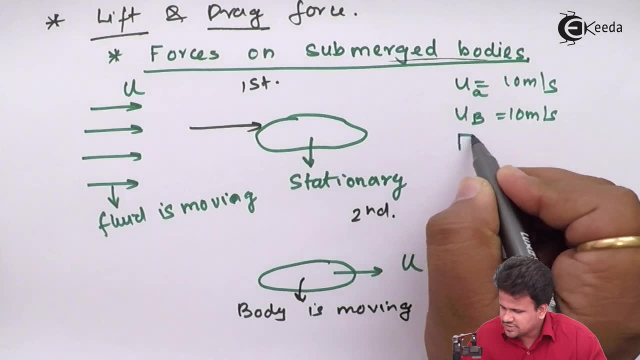 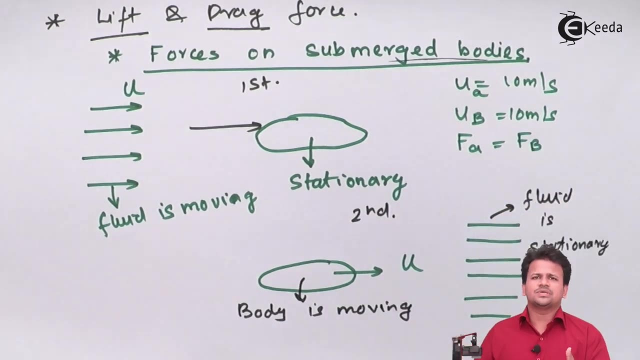 So the force exerted by the fluid on the body will be same as the body will exert the force on the fluid. That means the force exerted by the air will be equal to the force exerted by the body on the air. So it is an equal and opposite reaction over here. 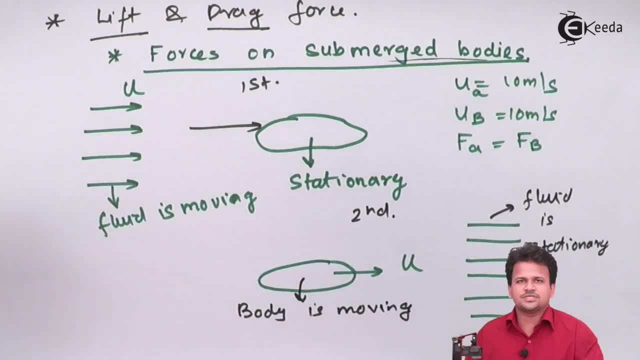 So these are the two conditions. The forces will be same whether the body is moving or the air is moving, Or the air is moving with the same velocity. So we have seen over here, there will be some amount of force which will be acting on the body. 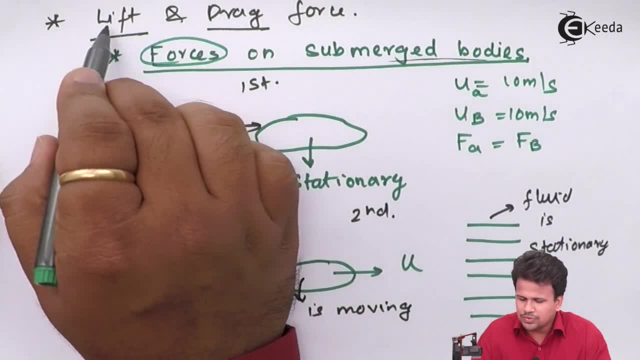 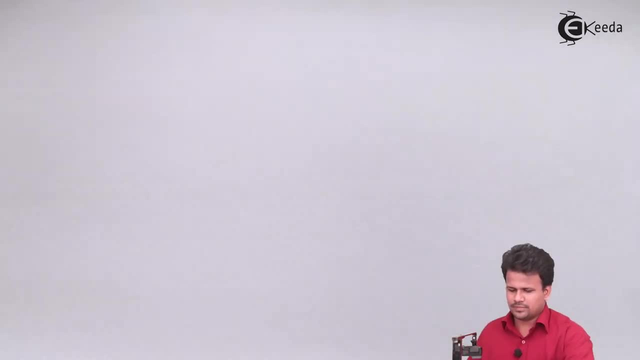 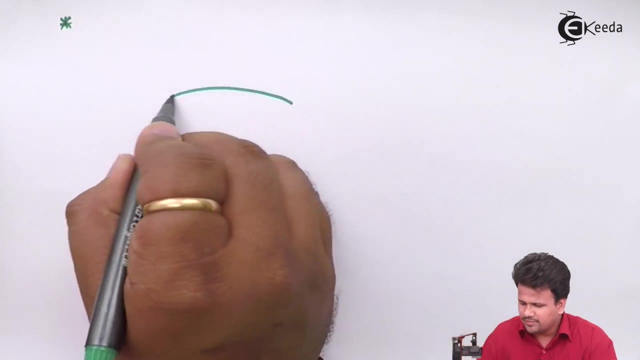 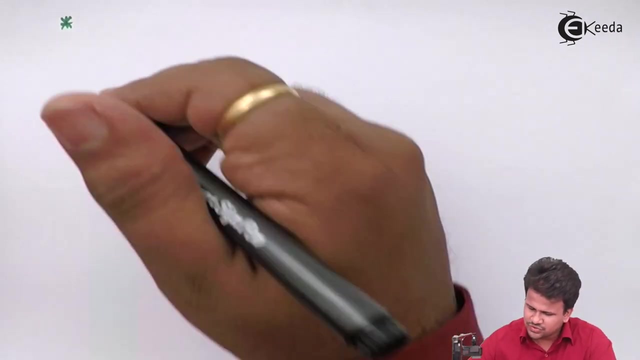 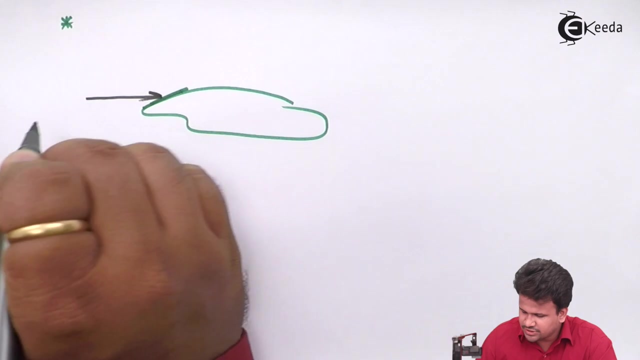 Now we have to differentiate this force into lift and drag. So let us understand what is lift and drag. To understand lift and drag, what we need to understand over here is a body which can be a random in shape. So this body, there will be a force which will be acting in the direction of the fluid. 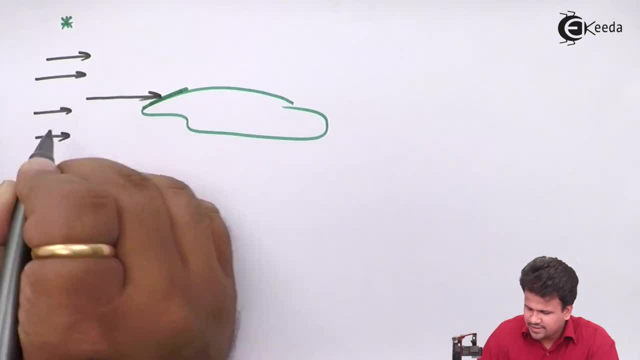 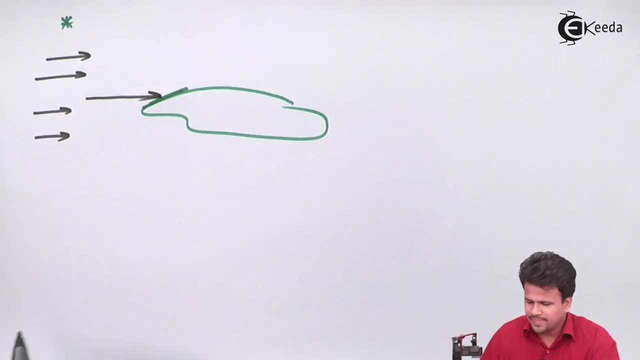 So if the fluid is moving towards right, there will be some force which will be acting along the direction of the fluid. This force will be called as the drag force. Now, what is drag force? Drag force will actually take the body in this direction. 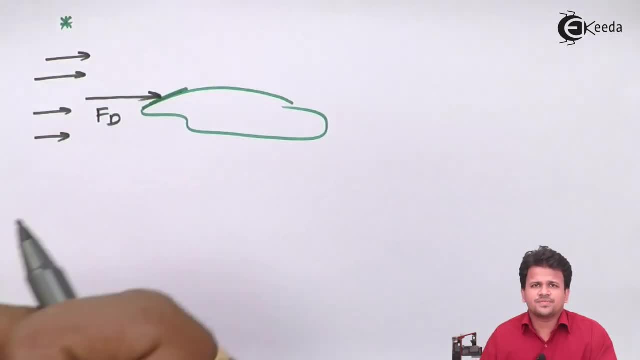 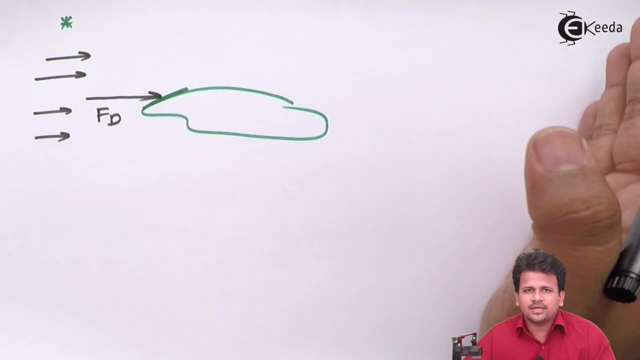 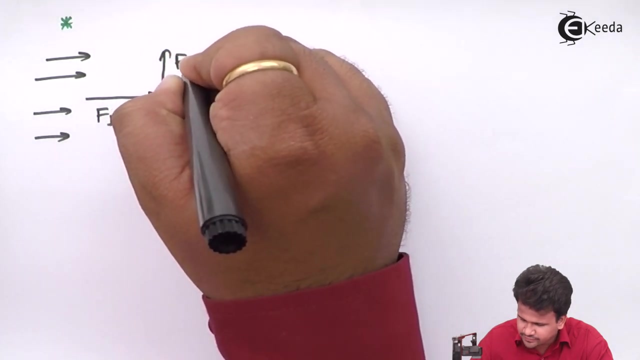 That is this air will have. if it has that much amount of velocity, If it is able to apply that much amount of drag force, then it will drag this body behind. Then comes a concept of lift force. Now, this is FL. Now FL is the lift force. 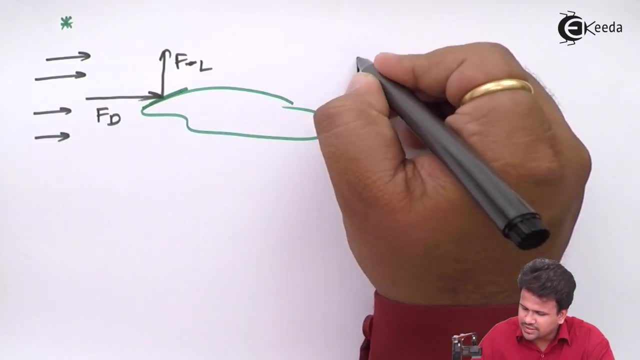 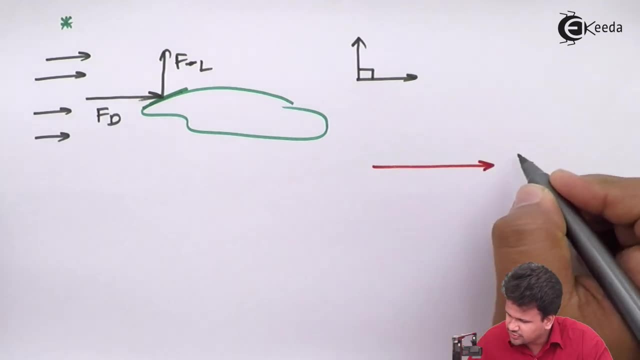 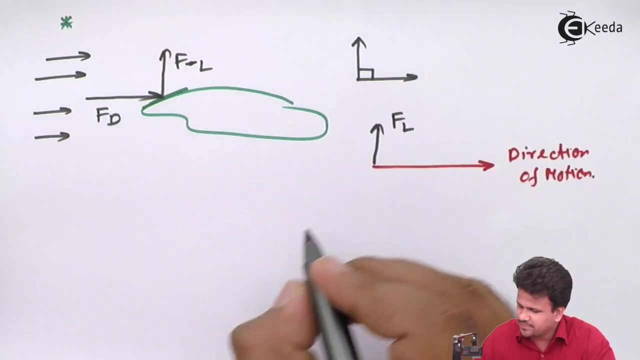 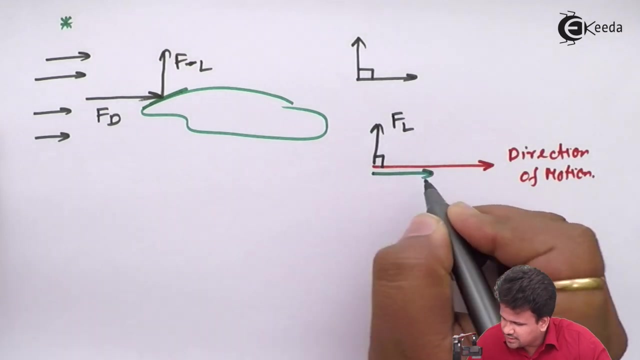 Which is perpendicular to the direction of motion. So we can draw it in this manner: If this is the direction of motion, Then the drag force is perpendicular. sorry, the lift force is perpendicular to the direction of motion, Whereas the drag force is parallel or along the direction of motion. 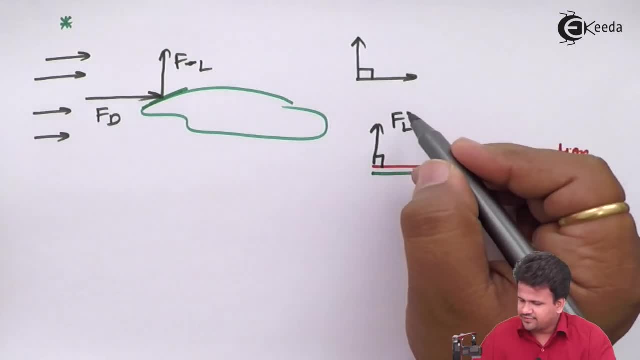 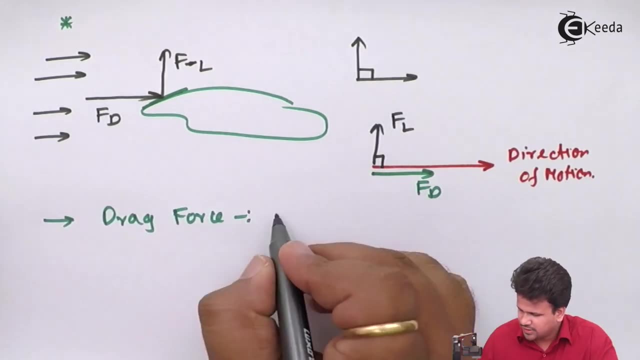 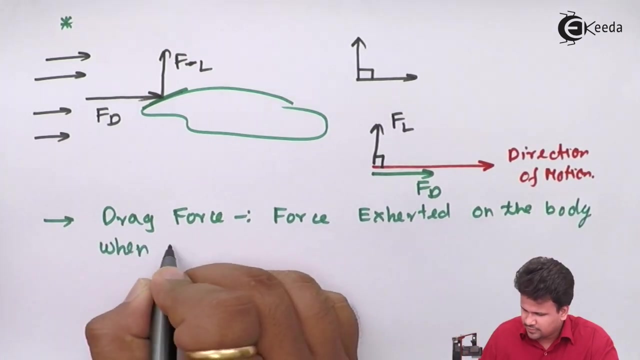 Now this drag force and this lift force we will just define over here. That is the drag force. 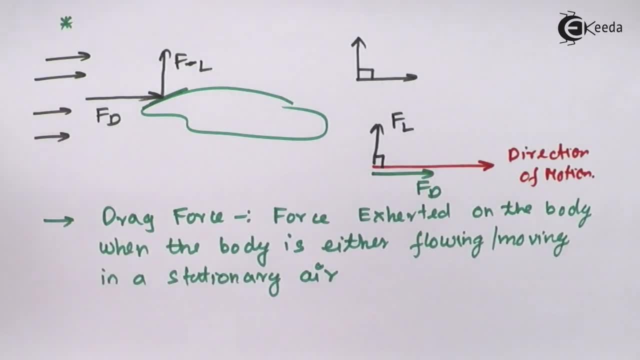 in stationary air, or the second condition will be: I it is, it is stationary. if the body is stationary, that is, the body and air is moving. So we have created the two conditions over here. 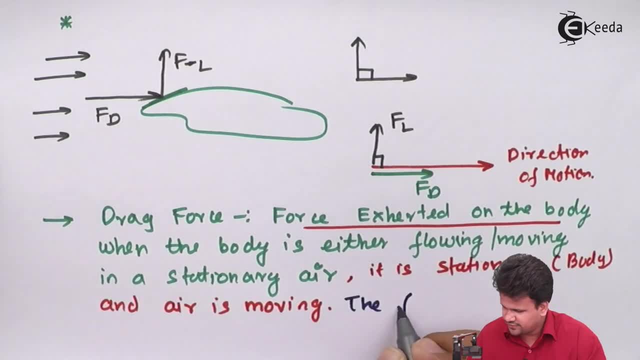 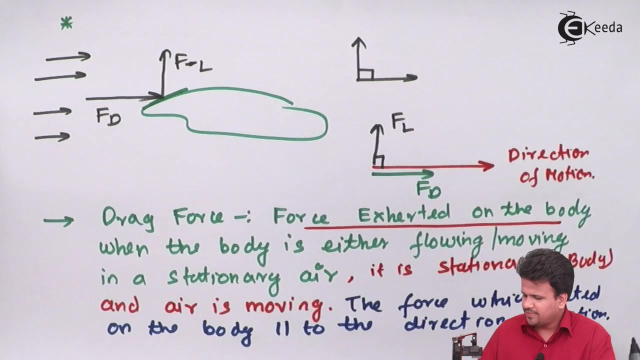 then the force, the force which is acted on the body, acted on the body parallel to the direction of motion, parallel to the direction of motion, will be called as the drag force. even if, if you do not specify this condition, then only then also we can define this as the force exerted on. 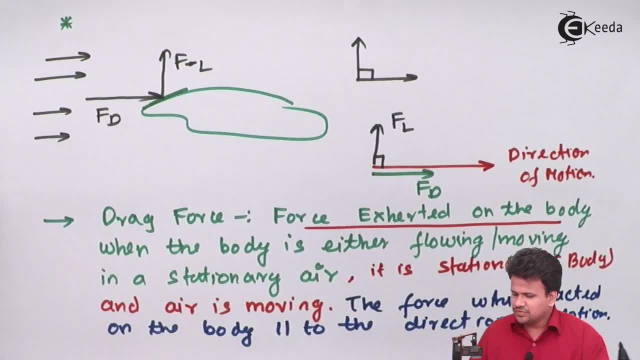 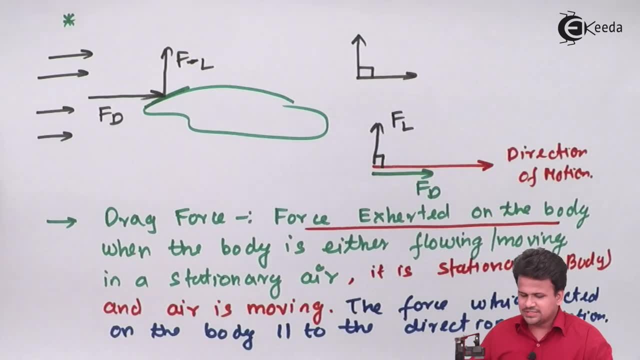 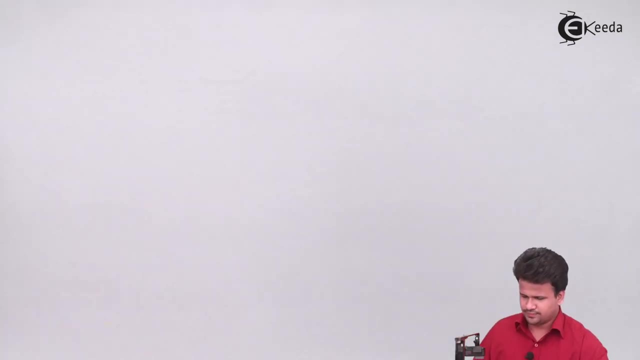 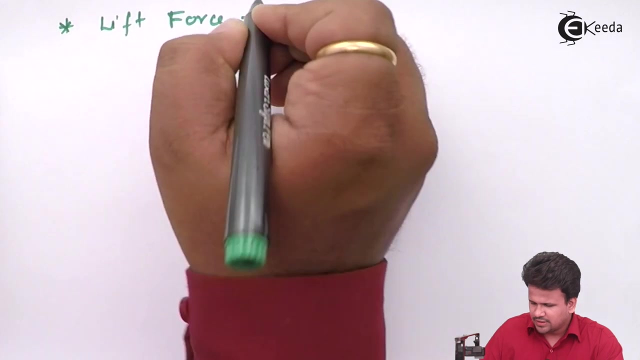 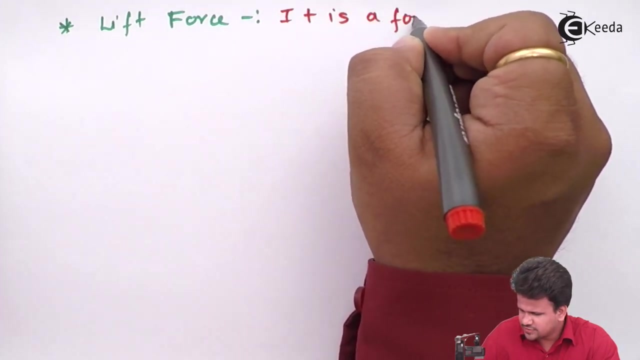 the body, when the force is parallel to the direction of motion, is called as the drag force. So now we have studied what is drag force, now let us define what is a lift force. Now for defining a lift force. it is a force we can write. it is a force which is acted on the body. 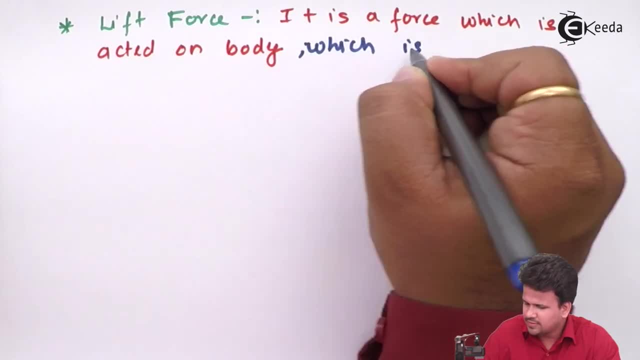 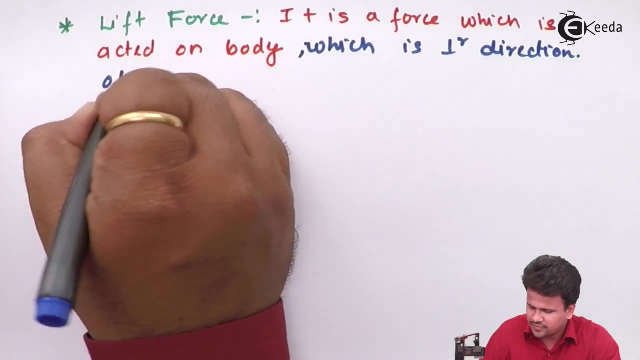 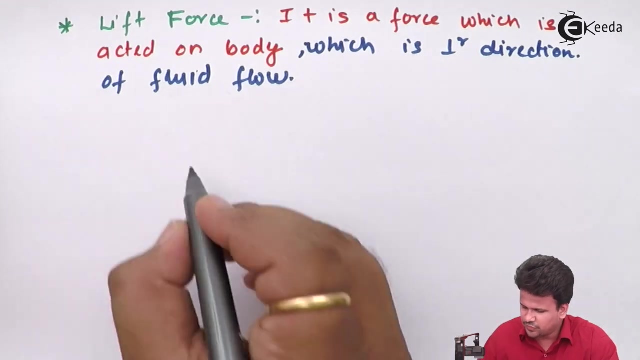 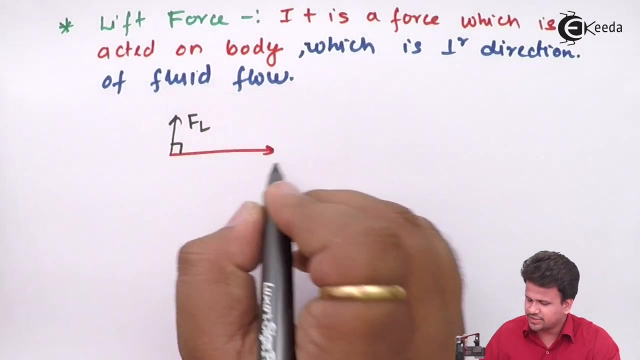 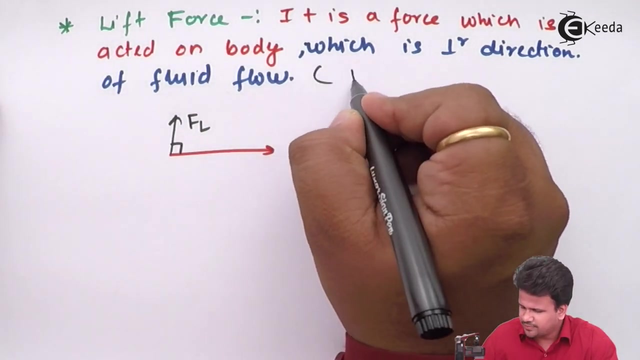 which is perpendicular to the direction of fluid flow. So if the fluid is flowing towards right, then the lift force over here will be perpendicular to the direction of motion. So that is called as the lift force, and then we can specify the condition: either the body, body is stationary, body will be stationary. 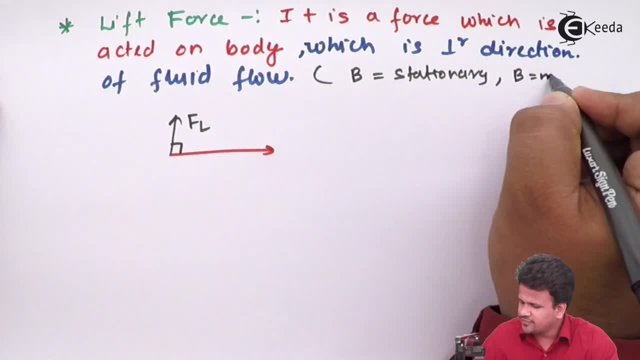 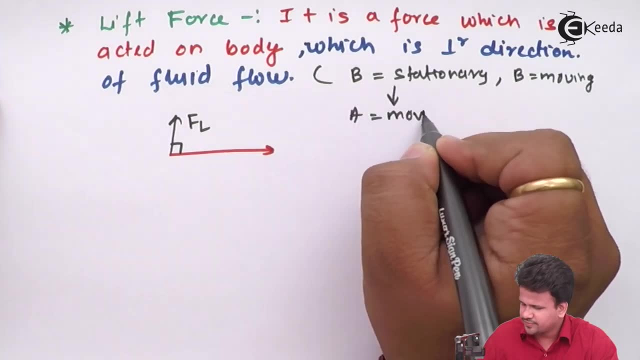 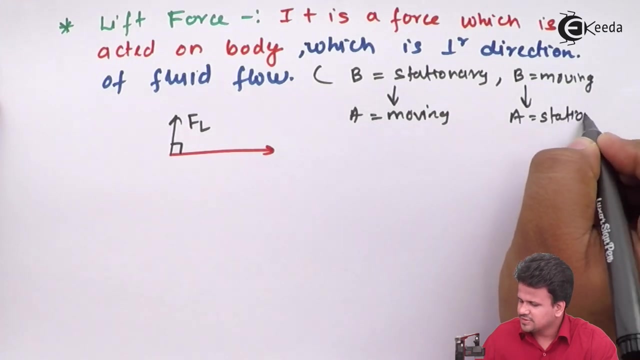 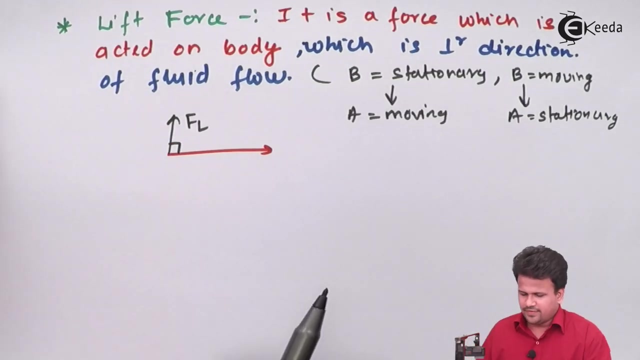 or body will be moving depending upon that. So if the body is stationary, the air is moving. and over here, if the body is moving, then the air will be stationary. So these are the two conditions which we have seen. So typically we can define both drag and lift force by just the direction of the motion. 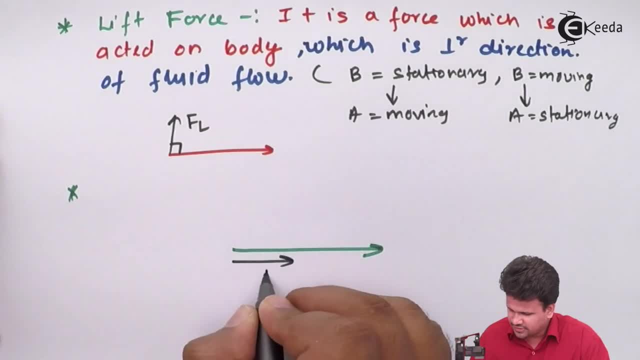 This is the direction of the motion, this is the direction of the drag force and this is the direction of the lift force. So now we have dealt with the drag force and the lift force. So let us just see where is this drag force and lift force is applied? So first we will. 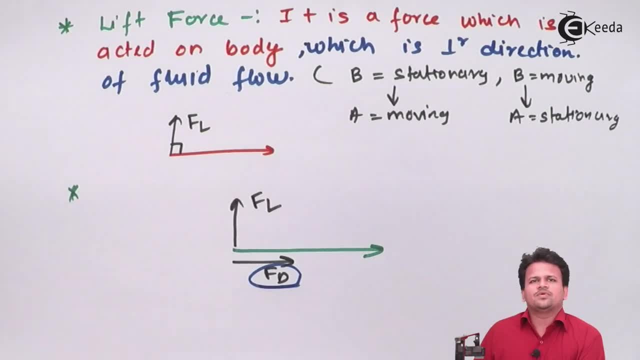 consider drag force. Now, the best example of drag force is a parachute. Now how a parachute is an example of drag force? Now, let us understand: whenever there is a skydiver, he is actually jumping from a very high altitude. Now, when he is jumping from a very high altitude, what? 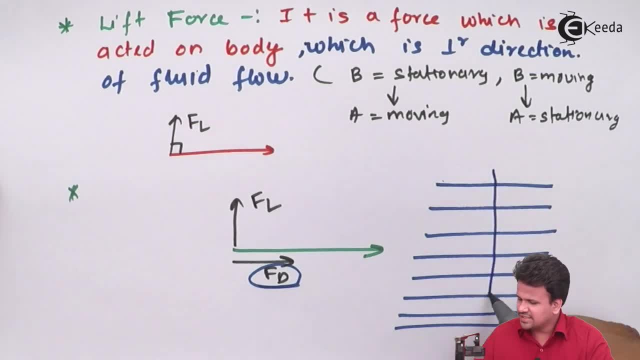 happens over here is he cuts through this various layers of the fluid. Now, while he is cutting this various layers of the fluid, he is actually jumping through this various layers of the fluid. what happens is his body accelerates to a maximum velocity. now in order. 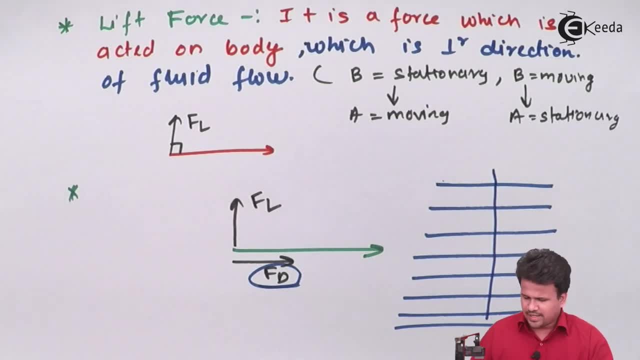 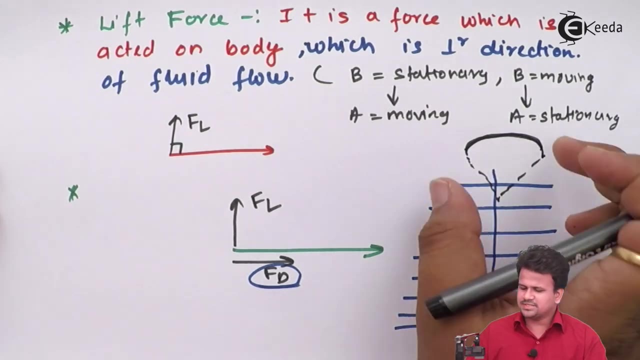 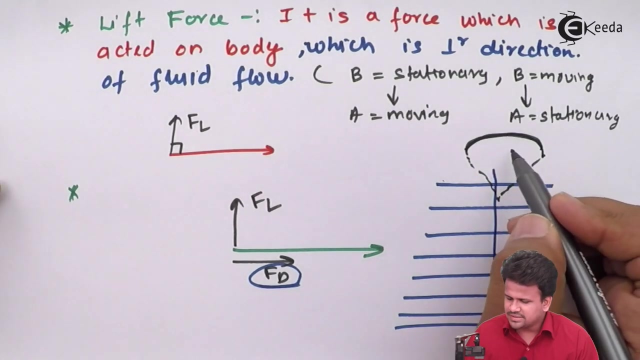 to reduce this velocity. what they use is a parachute. now, typically a parachute will be something like this: it will have a semi hemispherical, hemispherical surface, this hemisphere. what it does? it does that it traps the air. between that, it increases the area over there. if the area is increased, the amount of drag which is applied in is which is applied is in. 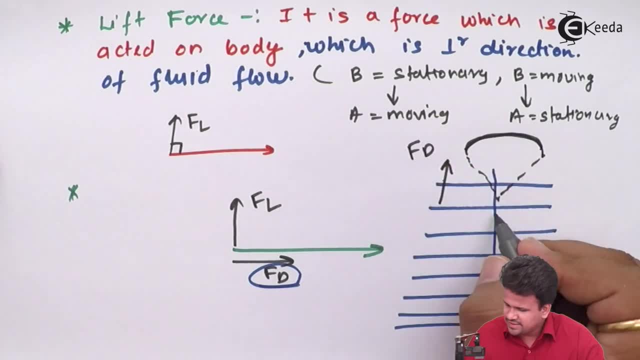 the opposite direction, that is, fd. this force which is coming down, this is due to mg, that is, the weight of the weight of the person which is going down. this force is very much high, but the drag which is on a person while he is coming down independently without any parachute is very less. hence to increase the drag. 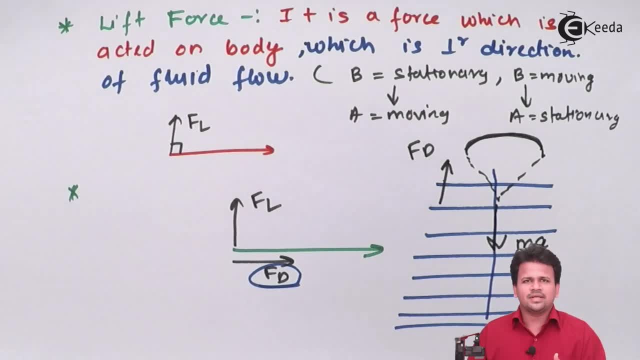 force and while he is coming down, he is accelerating. in order to control that acceleration, we use this parachute. now, when we use this parachute, what happens is we increase the drag force. so, due to this increase in the drag force, what happens is it can that free fall can be. 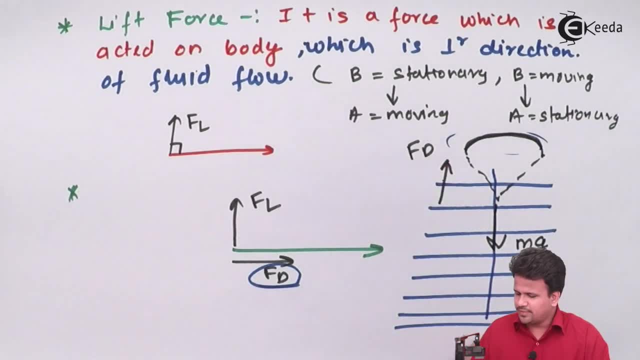 controlled, we can come down. we can come down to the surface very easily, but if in a case, there is no, there is no parachute, what happens is the drag force is very small and the person may come crashing down. we have observed skydiving videos. you must have seen that not all the skydivers are. 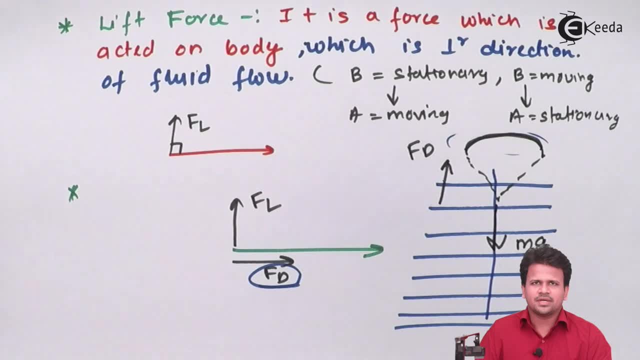 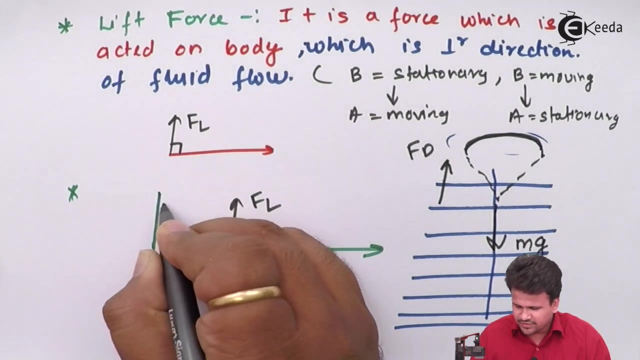 actually in a horizontal direction: horizontal. when they are in the horizontal direction, what happens is it increases the drag force which is applied on the body, thereby decreasing the acceleration by some amount. but if they are in the vertical direction, if it is the body, is the is in the vertical direction. 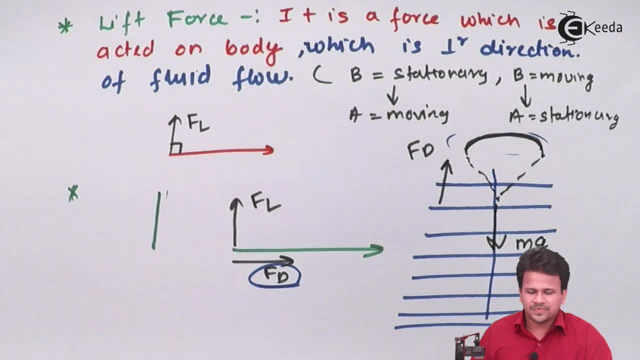 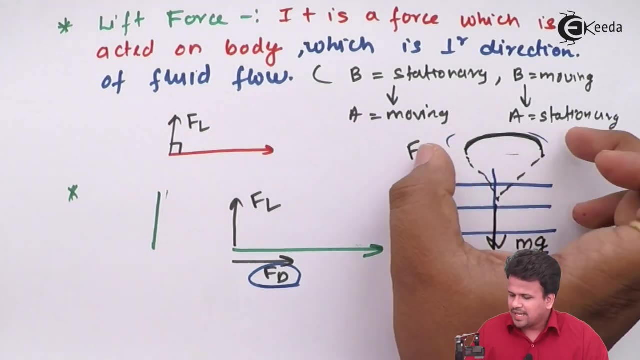 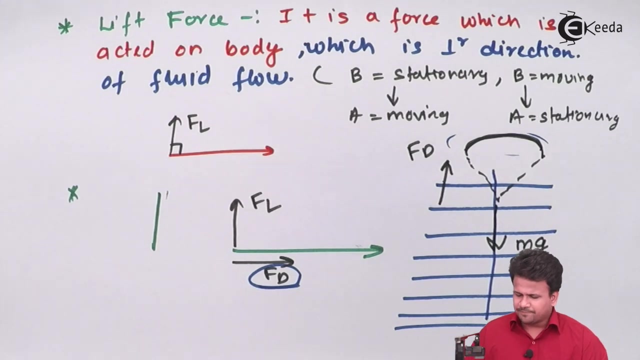 the drag force applied on the body is very small and due to the small application of a drag force, what happens is there will be more of acceleration. hence, what? hence, to increase the drag force, we increase the area over here and by increasing the area, what happens is the drag force increases and we can come down easily. now this track force is also. 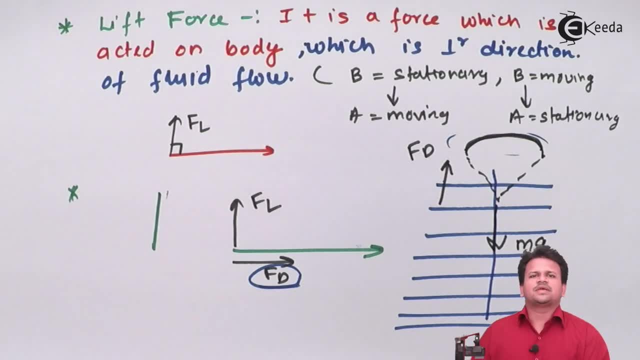 applicable in vehicles also. for example, we can consider a formula 1 vehicle. a formula 1 vehicle travels at a very high velocity. now we have observed that in formula 1 vehicle at the end there was an inch large�t chord and that in the other area there was an inch, like here and in the other. 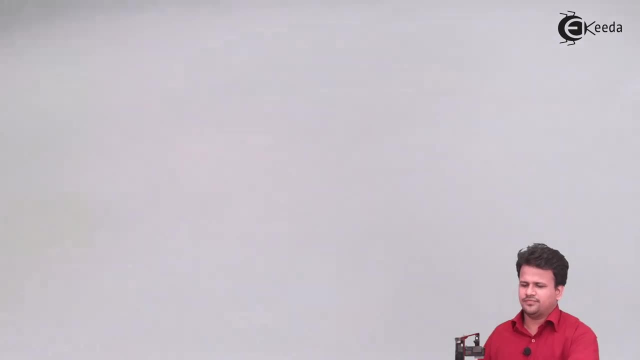 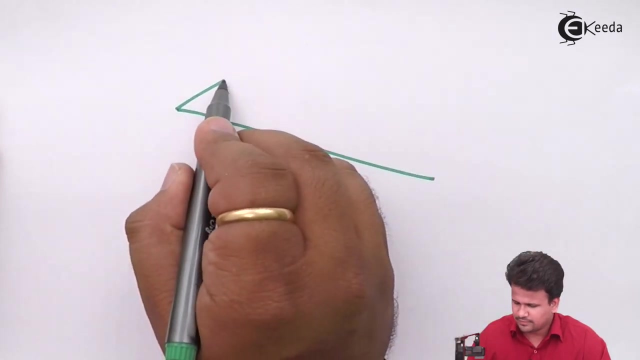 area, we have observed that the drag force of the vehicle varies, and so one thing to note here is that when we stand on a tree now, we can actually observe the damage happening on the trees right. so in products we have seen very similar to, you can observe that the drag force increases. 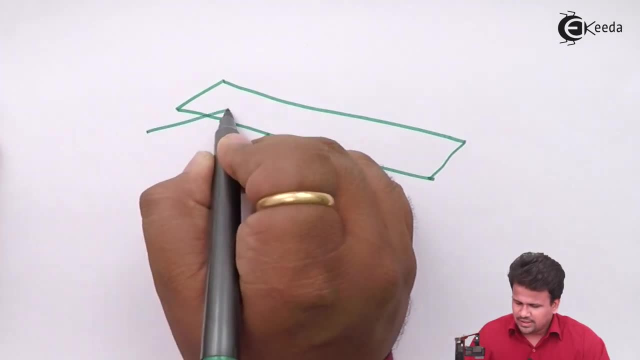 we don't get any impact. just remember, in this type of transport, the balanced일�nessMoments. you can observe they are the same, so the same in the other direction. we have long. if it looks like a curve, it will not have much displacements, the pressure will. 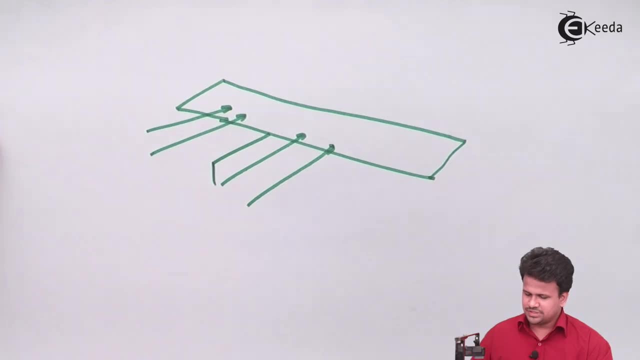 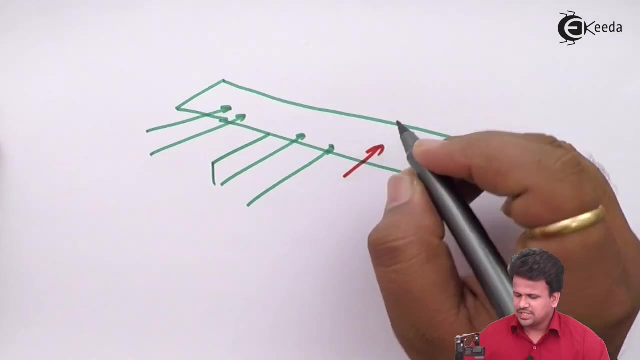 be high, while the g eine sign is great. you observe a short period of time, the distance between these Name applied over here. one forces will be a drag force which will be along this direction. the other will be the lift force, but since it is downwards, the lift force will go in the 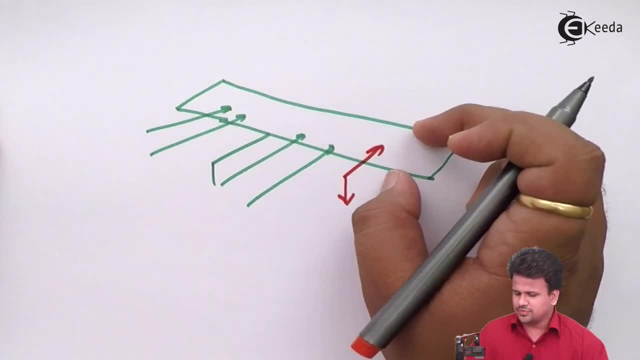 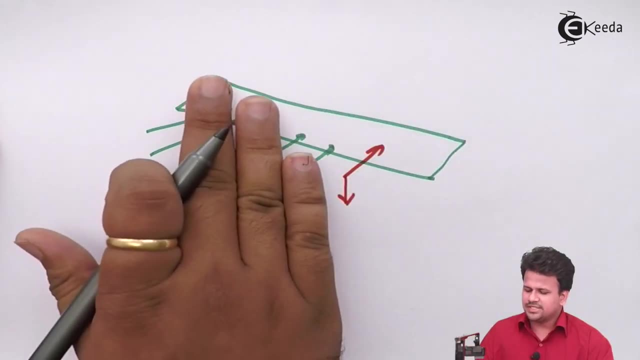 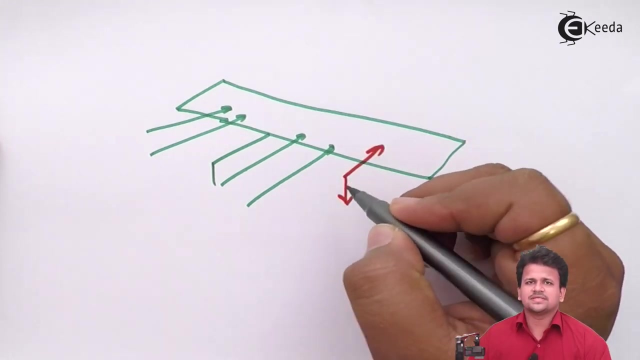 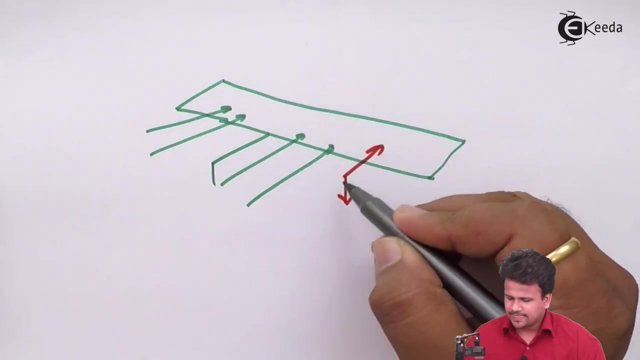 downward direction. This drag force over here is acted upon, this in formula one vehicle. now, this is made sure that this drag force is as minimum as possible, but the lift force over here is as maximum as possible. Now, what happens over here? now, this drag force is minimum because the area of cross section. 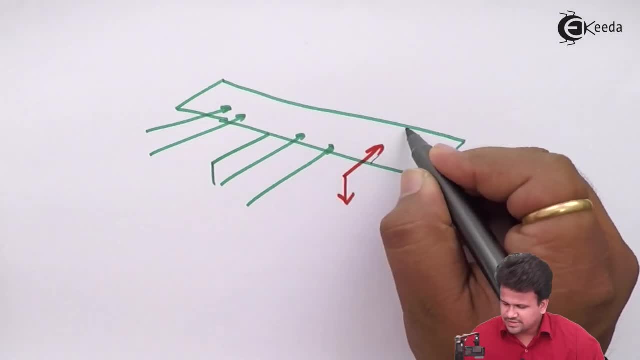 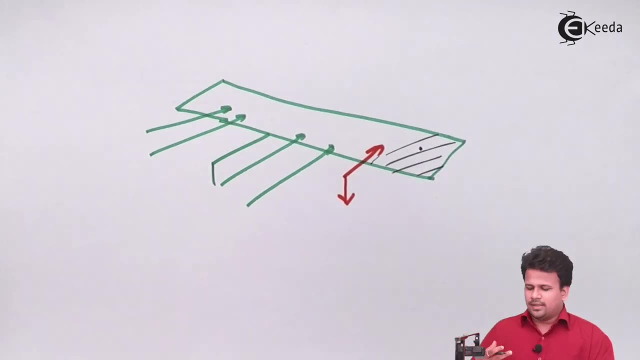 of this is very small, but for the lift force, this entire will be the area of cross section. Now, this area of cross section enables the body to be on the lift force. Now this drag force will be on the surface, or else it may lose the contact with the entire. 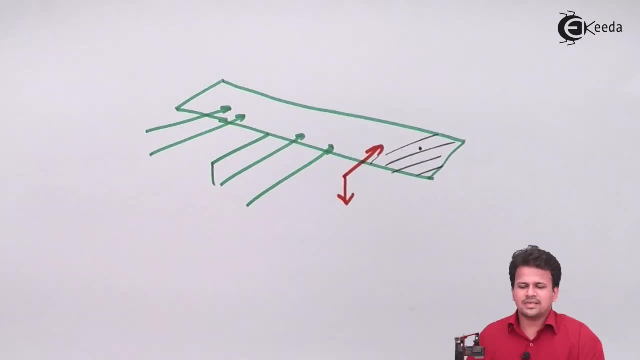 surface. So I hope you have understood what are real life examples of drag force and lift force. Now another example of lift force we can take is flying of a kite. Now, when we fly a kite, what happens is there are two forces which we are making responsible. 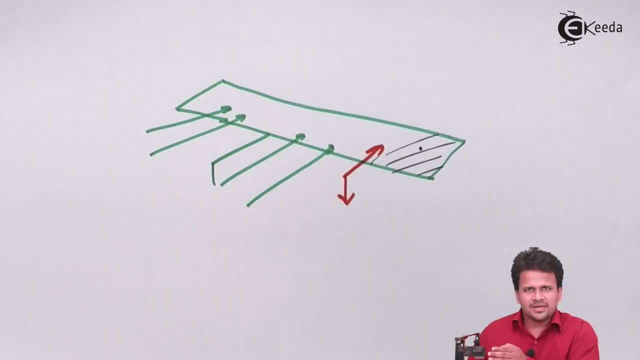 for That is first, the wind will drag away the kite force From one place to another place, But the lift force is applied by the individual, by lifting the entire kite in the upward direction. So individual provides a lift force and the air provides a drag force, due to which the 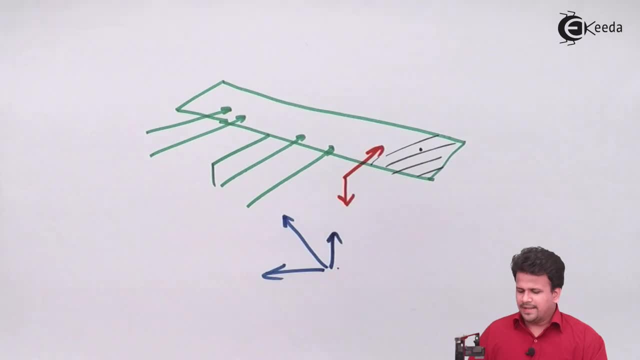 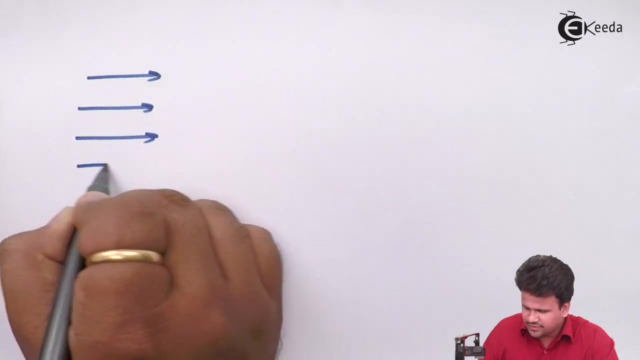 kite flies in the upward direction. Now the direction can be controlled by the observer or an individual, depending upon in which direction he has to take the kite. So now let us study this drag force and lift force in detail. Now for this, we will consider the air which is moving at velocity u, and there is some. 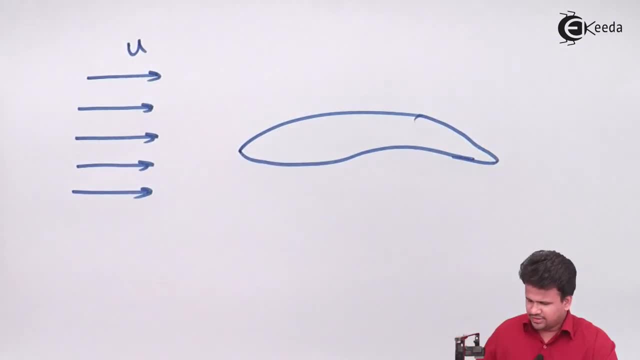 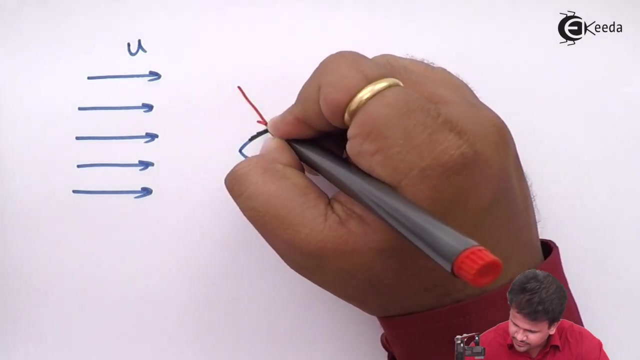 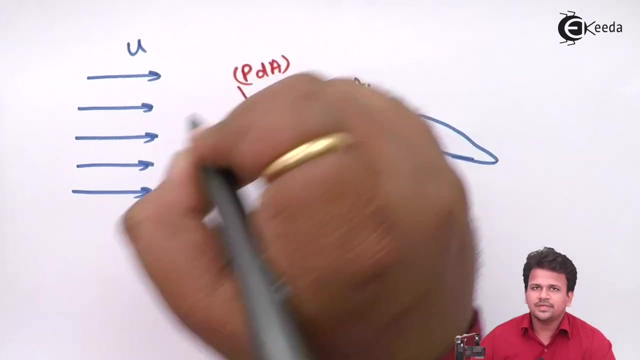 random body over here On this body. let us consider area dA. On this area dA, there will be some amount of force which will be acting perpendicular. This will be called as the pressure force. This will be the pressure into area of cross section will be dA. 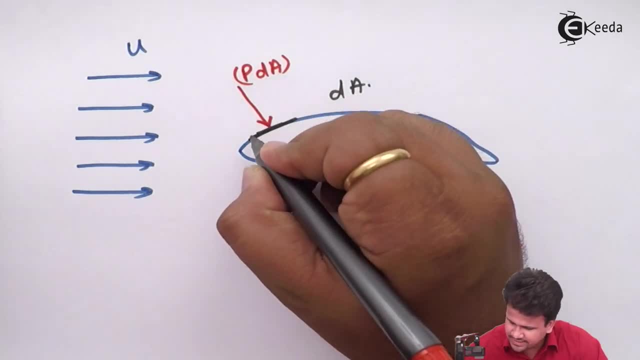 So this is the pressure force and the force which is acting along the direction or pressure. So this is the pressure force, So this is the pressure force, So this is the pressure force and this is the pressure also acting between area dA and area dA. 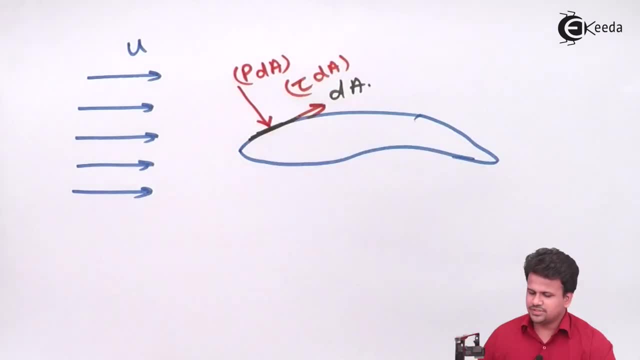 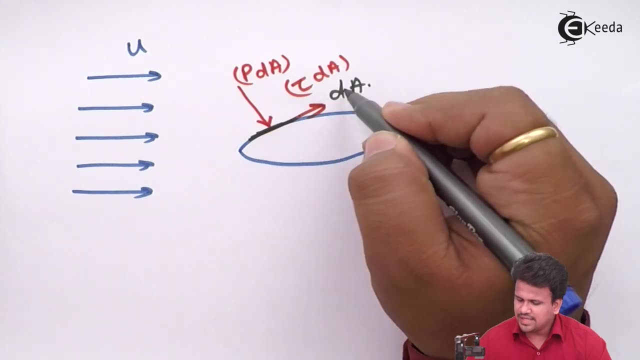 This is the pressure force opposite area u, and this is the pressure force which is acting in parallel to the area, is equal to tau dA. So this is the shear force. So this force, pressure, is perpendicular to the surface and tau into dA is parallel to. 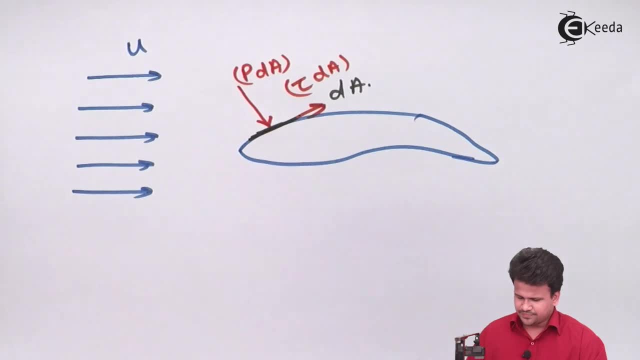 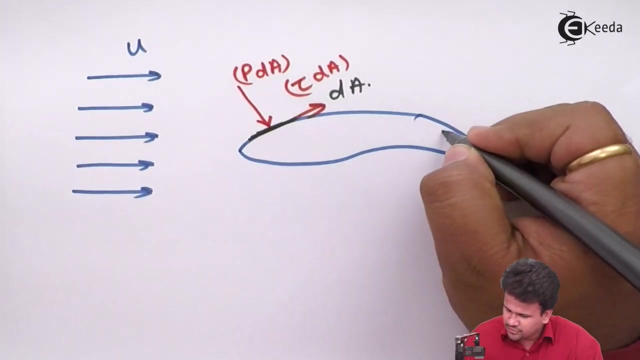 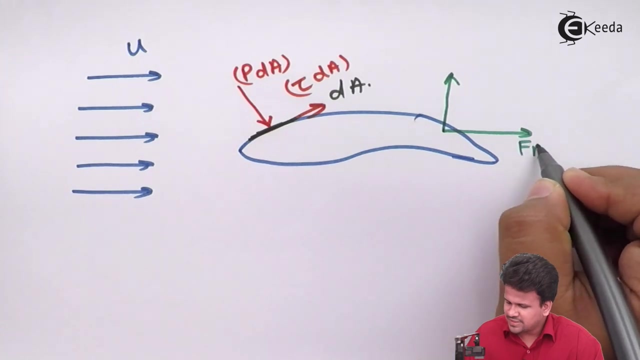 the parallel or along the surface. Now, our lift force is typically defined as the force which is perpendicular to the direction of the flow. if this is the direction of the flow, then the lift force will be upwards and the drag force will be towards right. So this is the drag force, this is the lift force. Now let us consider: 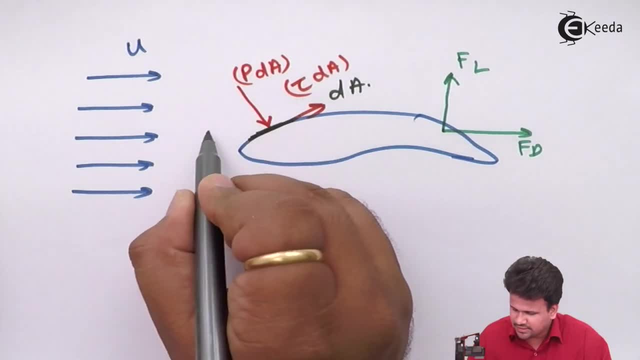 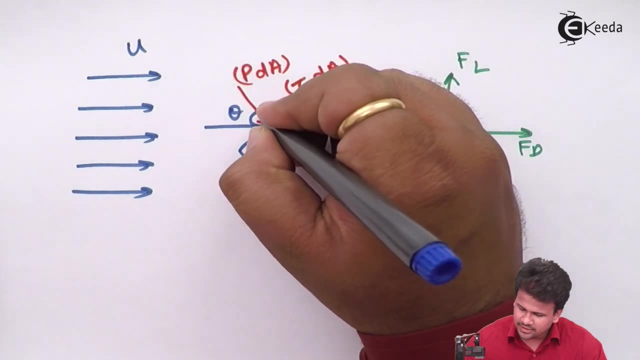 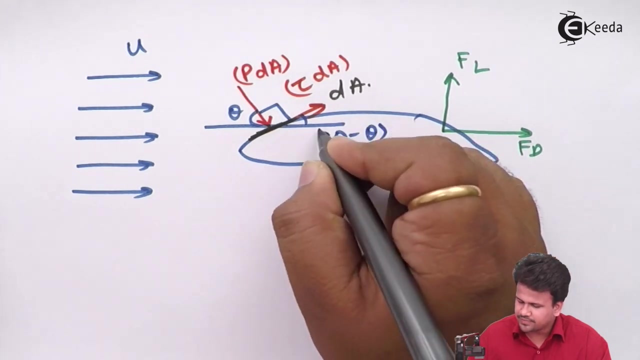 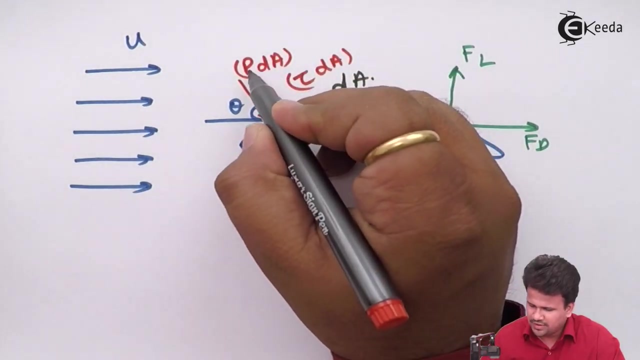 that this area or this entire thing makes an angle of theta with the horizontal, and the angle between pressure force and the shear force is 90. Hence this angle over here will be 90 minus theta. So we have seen both the angles over here, So now we have. so we have over here the pressure. 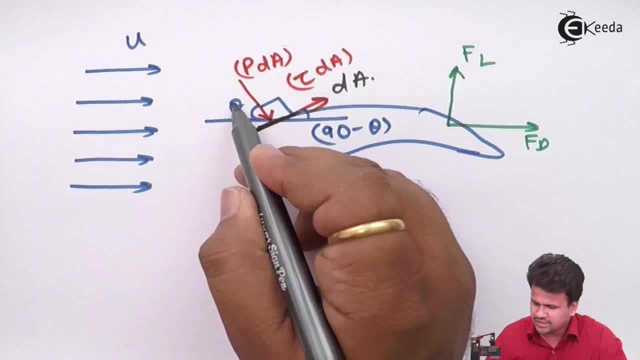 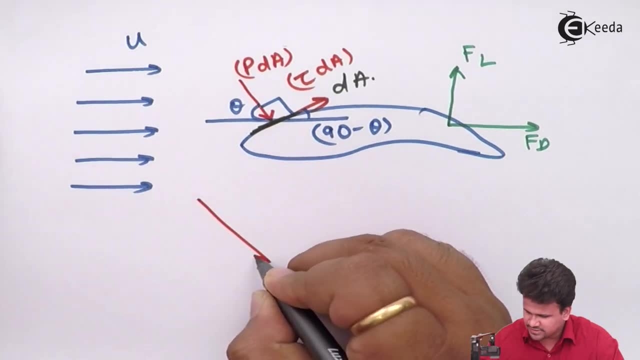 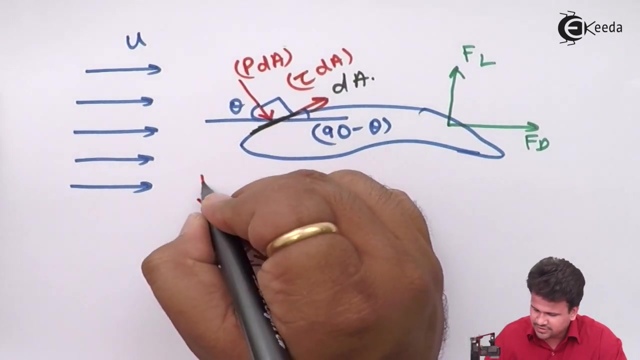 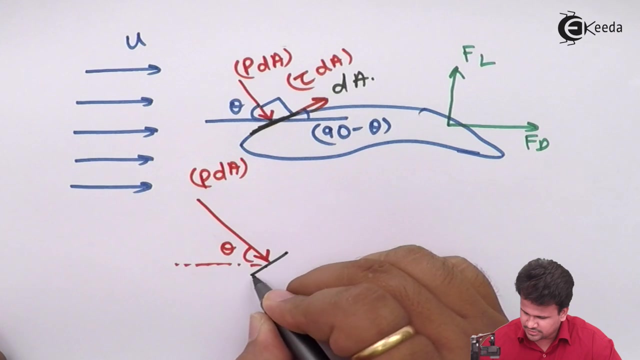 force and shear force which are making an angle of theta with the horizontal and 90 minus theta with the horizontal. So if we draw this separately, this is the pressure force. with the horizontal it it is making an angle of theta. So this is a P into dA on the area which is in this direction. 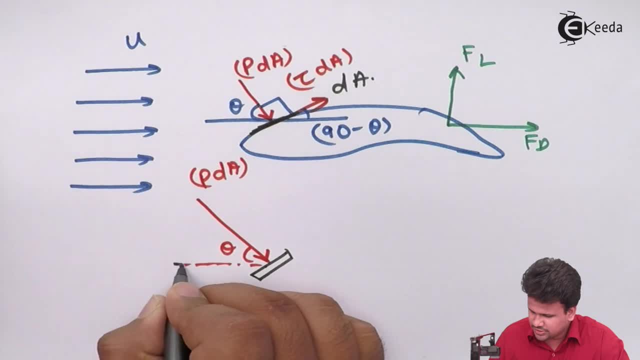 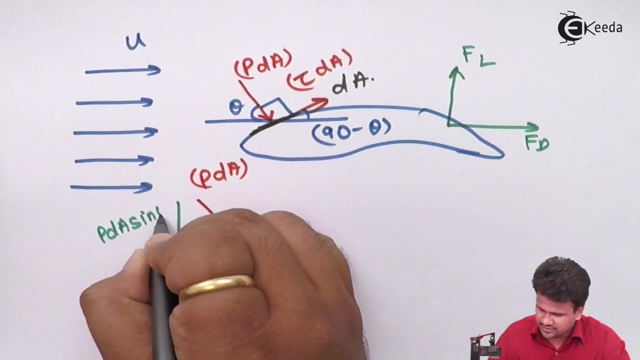 So its component will be: the horizontal component will be P into dA cos of theta, and the vertical component, which will be in the downward direction, will be equals to P into dA sine of theta. So we have seen both the components, that is, P into dA cos theta and P. 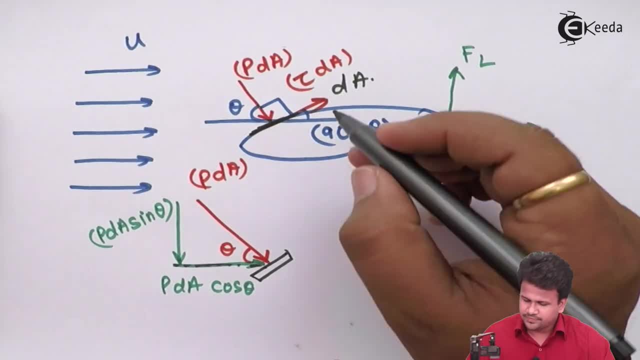 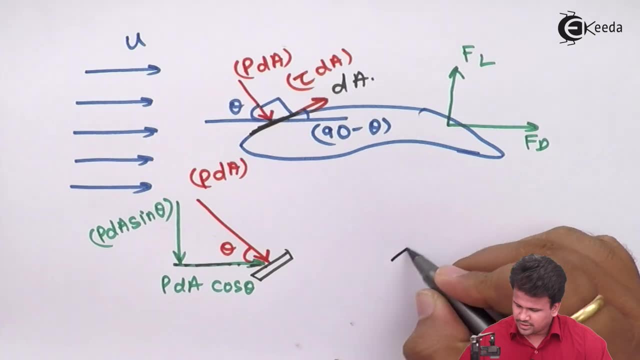 into dA sine theta. Now let us see about this force over here that is T into dA, tau into dA, to be precise. So now this force is along the surface of the area. that is tau into dA. Now this is making an 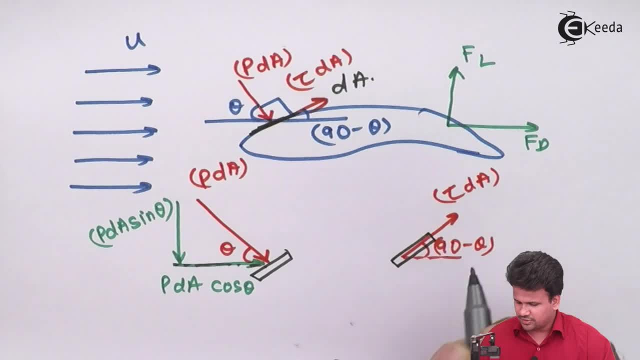 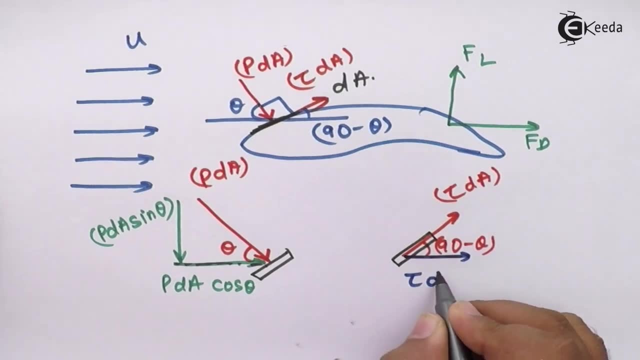 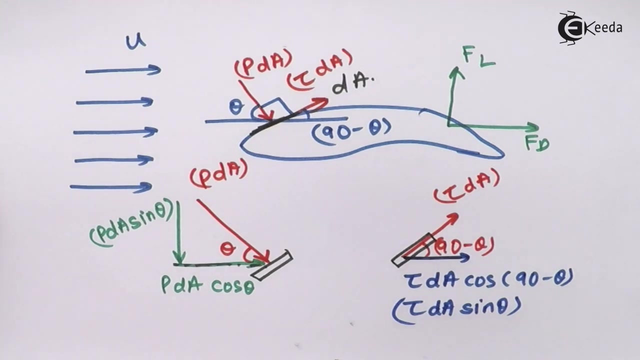 angle of 90 minus theta with the horizontal. So its horizontal component over here will be equals to tau into dA, cos of 90 minus theta. Now we already know cos of 90 minus theta is sine theta. So tau into dA, into sine of theta. So this is the force along horizontal direction and the force. 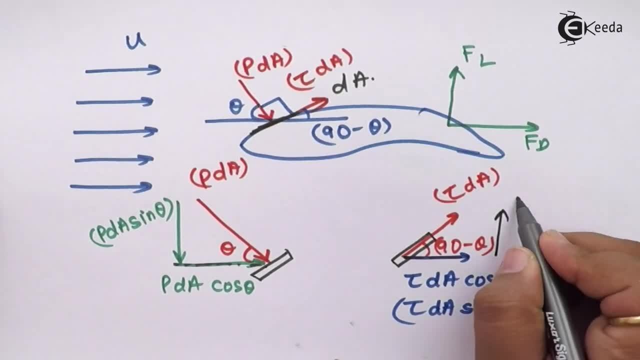 along vertical direction will be equals to tau into dA sine of 90 minus theta, which is equals to tau into dA cos of theta. So now we have seen both the horizontal and vertical forces. Now, using this analogy, we can write what is the drag force and what is the lift force. Now 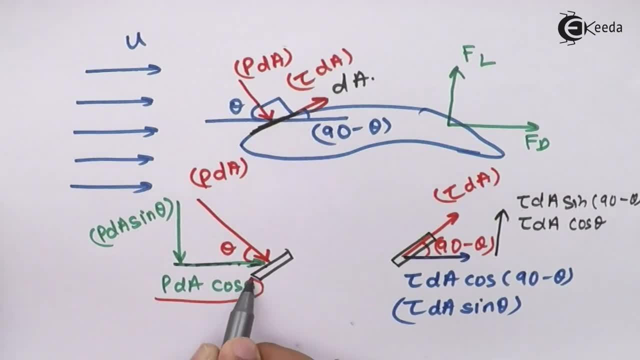 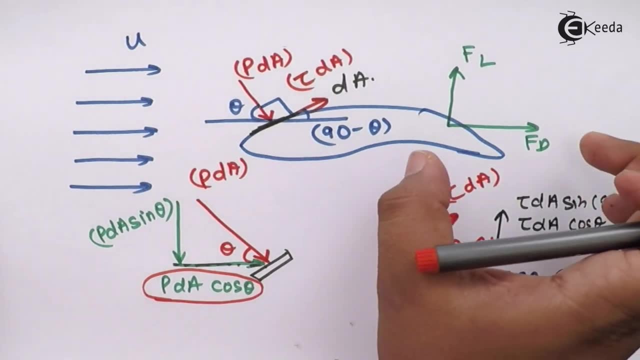 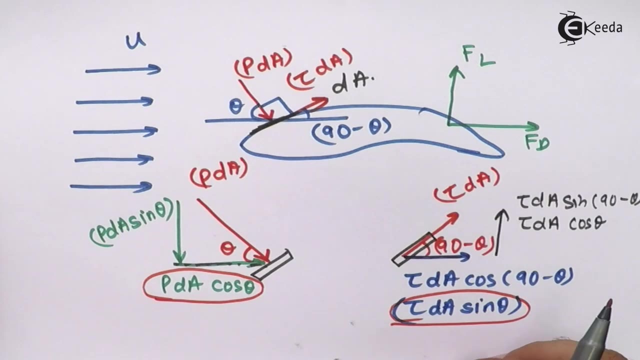 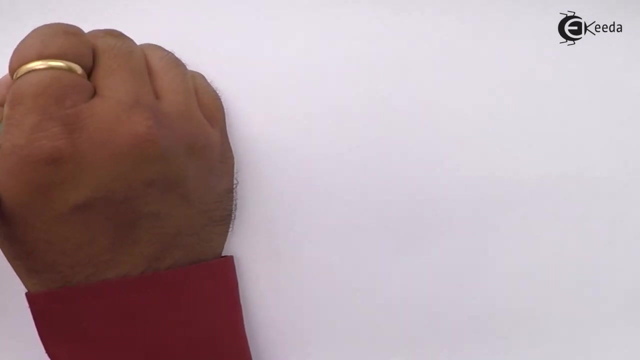 drag force, which is in this direction. So another value that we have is without the loss constant, or the loss constant is the force acting on the body, and that is from t to dA. that is, pa cos theta plus tau into dA sine theta. So addition of this will be in the direction of drag force. So this is the 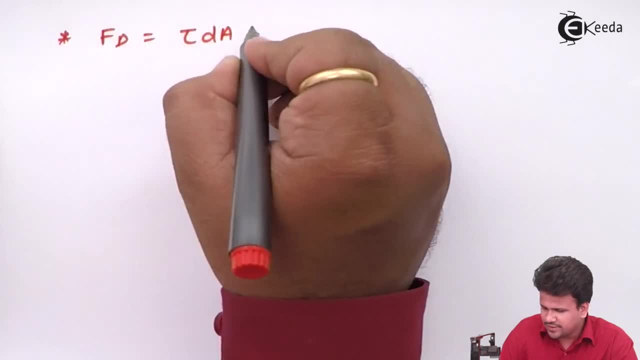 drag force which is acting on the body. So let us write down this part, So the net drag force can be written as: Fd is equals to tau into dA sine theta plus dA sine theta minus dA. This is also needed. Well, the moment of infinity goes to ay and we have to see which one'll be acting on the body, and that should be the top. 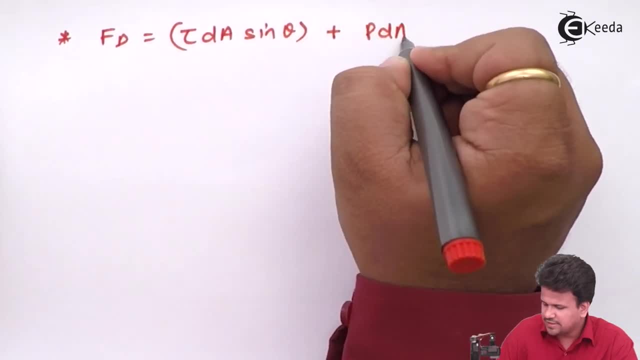 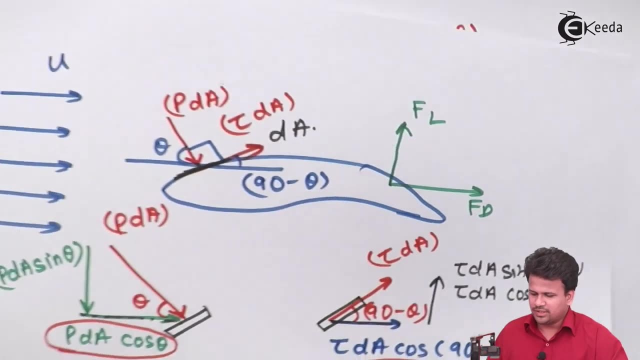 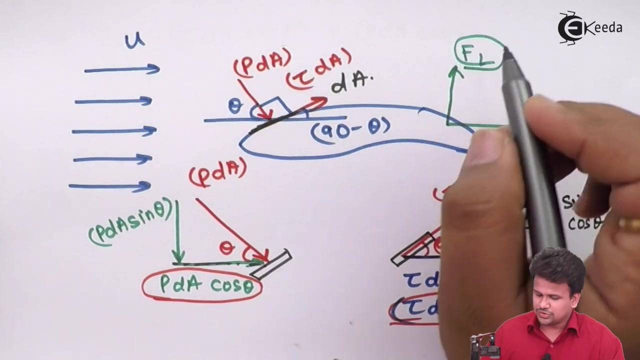 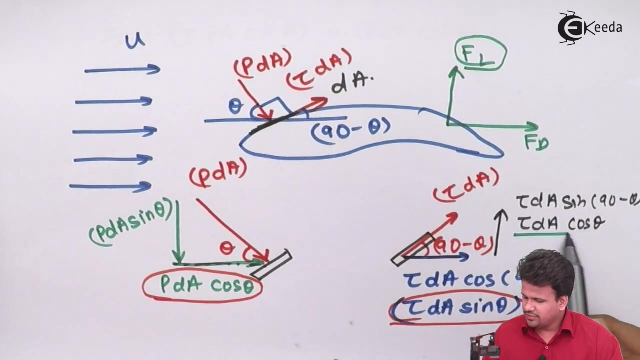 plus P into da, into cos of theta. Now next we will write about lift force. Now, from the diagram, if we can see, the lift force is perpendicular to the direction of motion. So there are two forces which are along this direction over here, that is, tau into da cos theta and P into da sin. 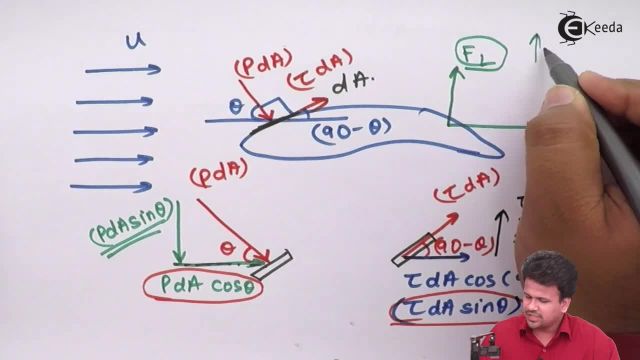 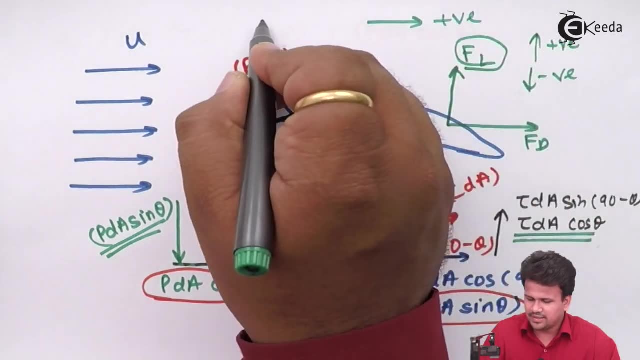 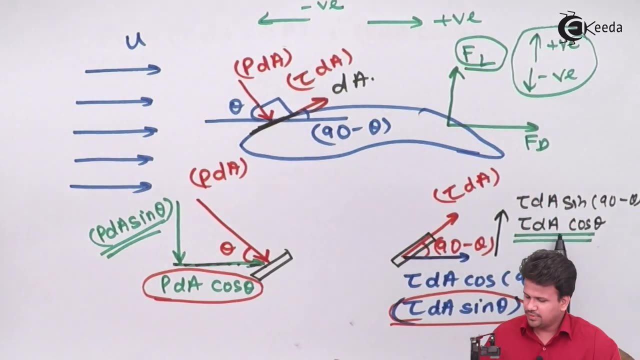 theta, But if we consider all the forces which are going upwards as positive and downwards as negative, Similarly, right hand side should be positive and left hand side should be negative. Applying this concept, we can write this as tau into: da cos theta minus P da sin theta is equals. 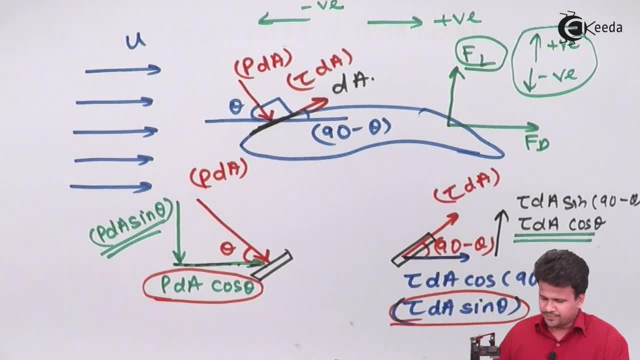 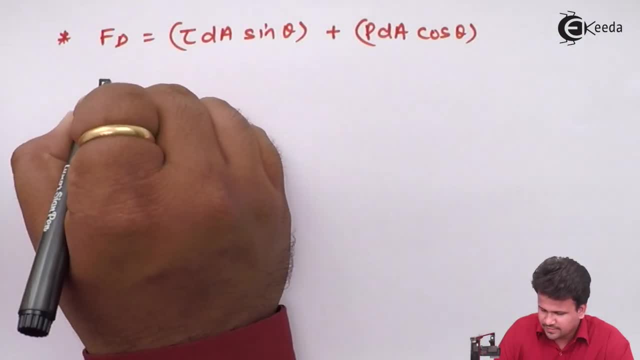 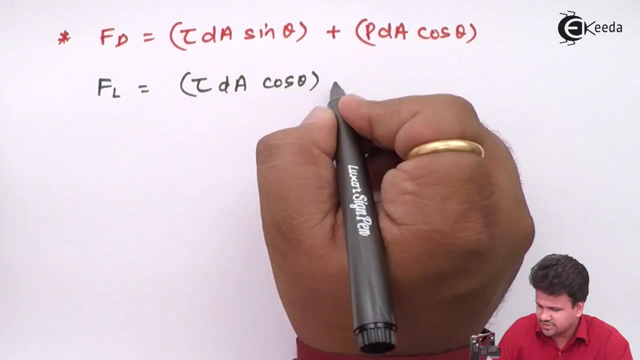 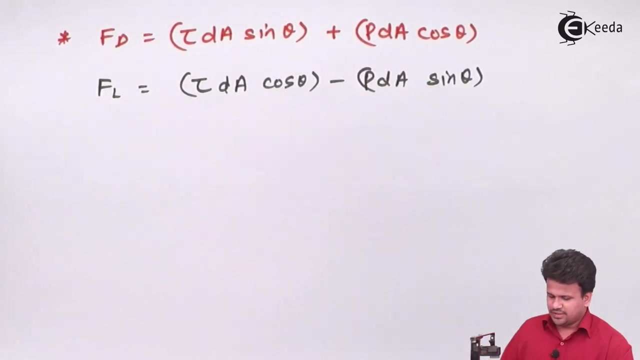 to the lift force which is acting on the body. So let us write down this part over here, That is: lift force is equals to tau into da cos theta, which is positive, minus P into da sin theta, which is negative. One more thing: if we have to calculate the net force, 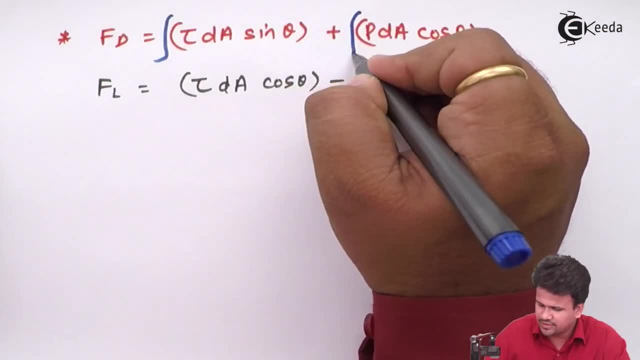 that we have to integrate this over that entire area. So we have to integrate over that entire area. So this is gonna be the lift force that we have, tooru, the lift force Now, етров will be given as tau D into da cos theta. Now everyone can see this here. Remember we have 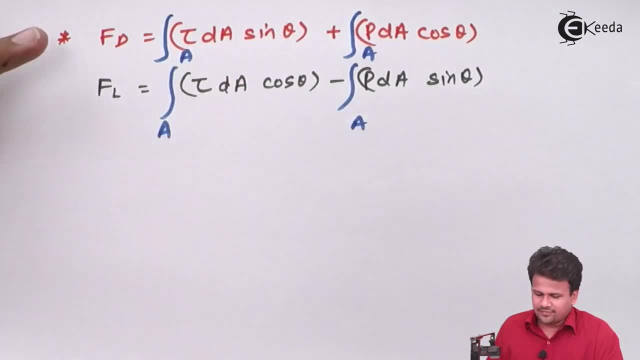 So this is gonna be the lift force that we have to rokuand it into the negative slope And, of course, tattoo as a Economics of grazing over here. then this will be sub duca relation for this point Now area. So that will give us the net drag force and lift force. Now we have seen what is the net. 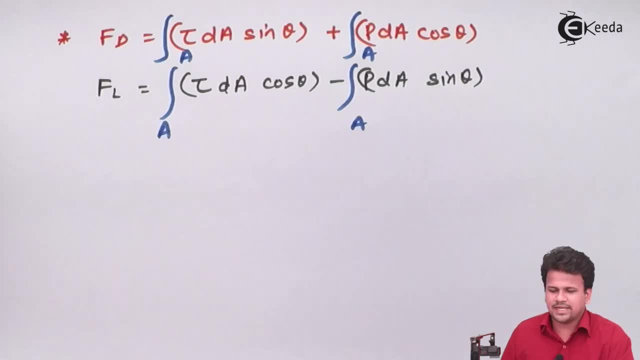 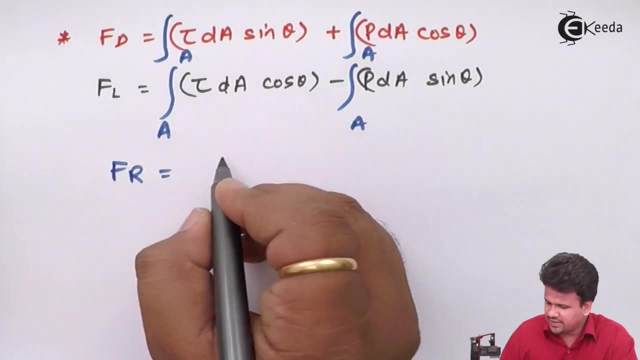 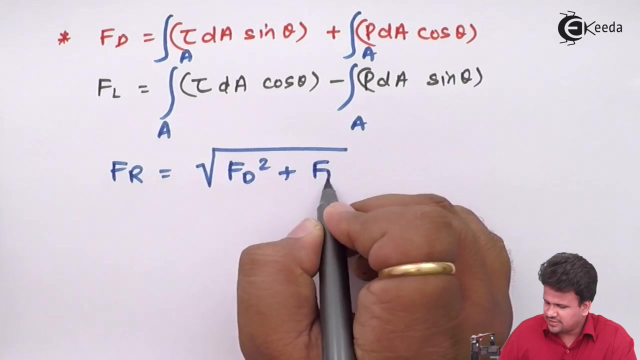 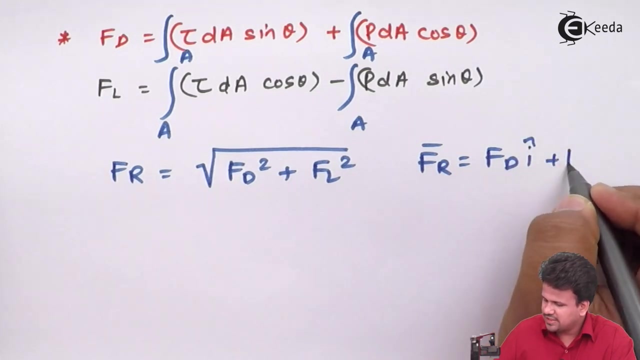 drag force and lift force for a body which is inclined at an angle of theta. Now the total force, F, resultant in vector form can be written as square root of F d square plus F L square. In vector form, F? r will be given as F d i cap plus F L, j cap and theta will be given as tan. 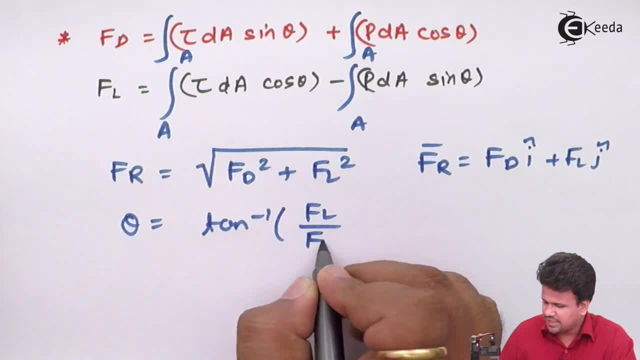 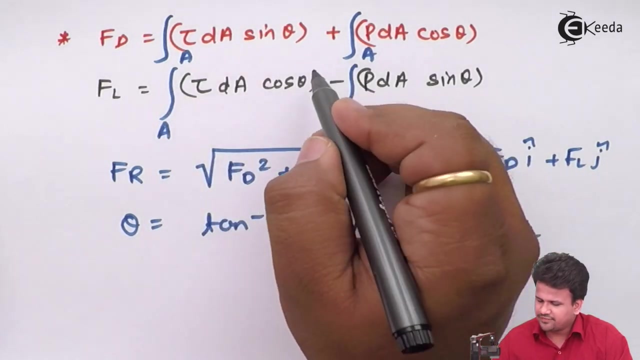 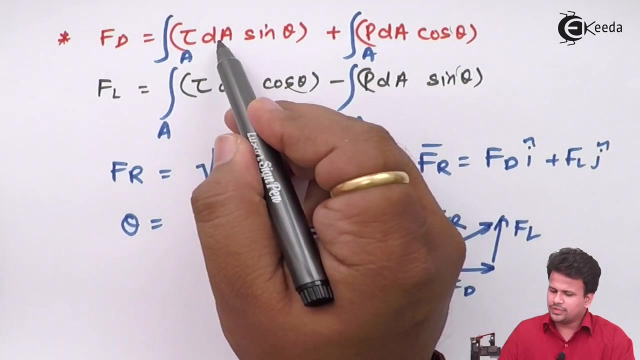 inverse of lift force upon drag force that can be given by this triangle, F d, F, L and F? r. This angle will be theta. Now, what is important thing over here? that in this part the lift force and drag force is entirely controlled by these quantities. that is theta. The area is going to remain constant. 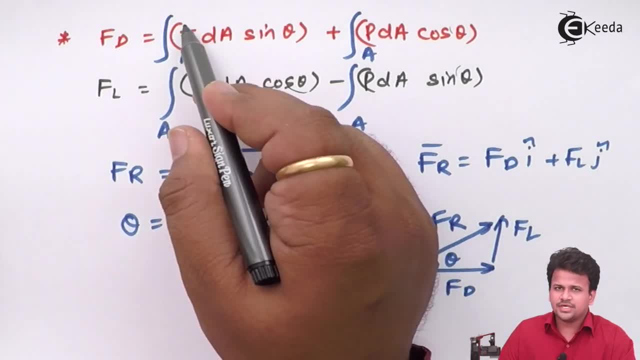 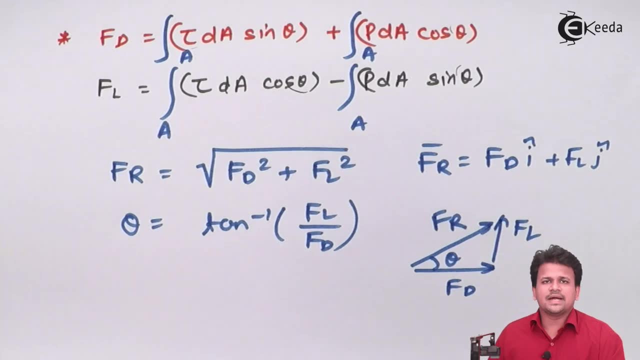 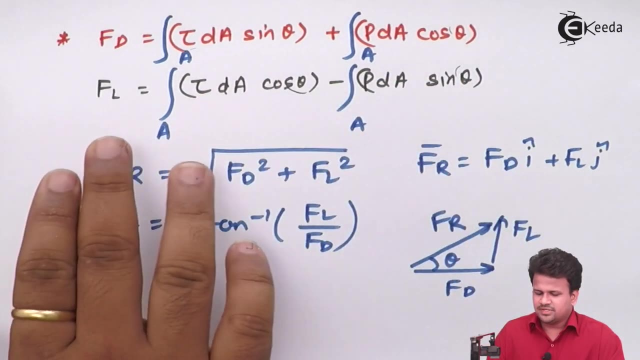 the drag is going to remain, the shear is going to remain constant and the pressure is going to remain constant. What things are changing over here? that is value of theta. So let us understand, let us write, let us take this equation and we will keep this force as function of theta and we will calculate. 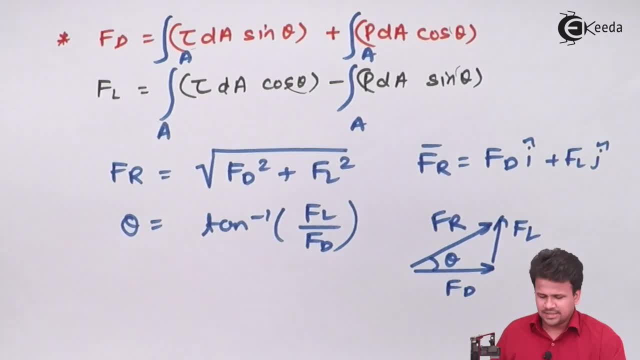 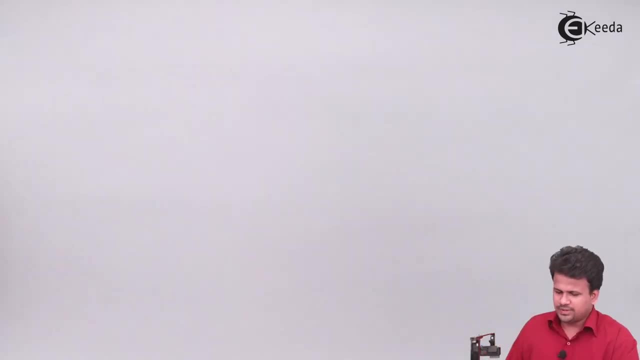 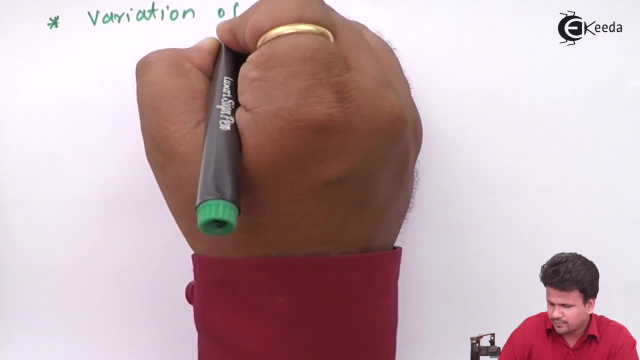 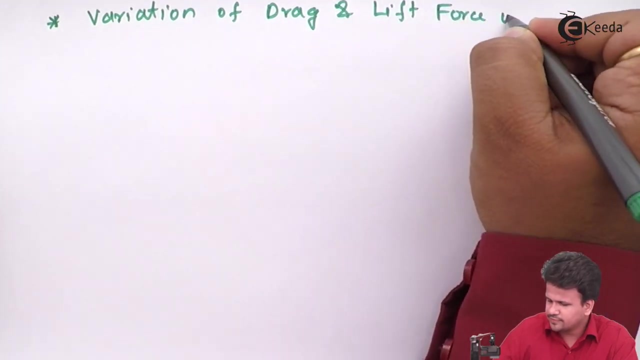 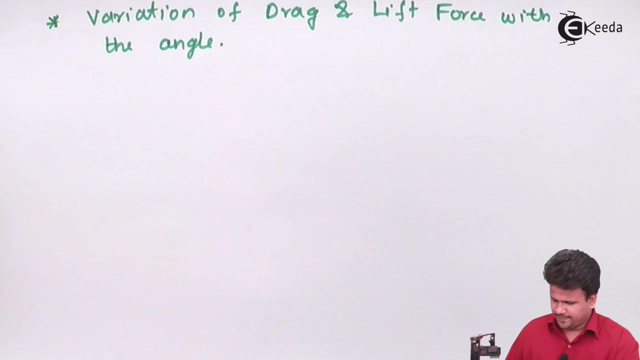 what happens when the angle is 0,? what happens when the angle is 90. Let us see variation of drag force and lift force with variation of and lift force with the angle. Now let us write down over here what is a drag force. 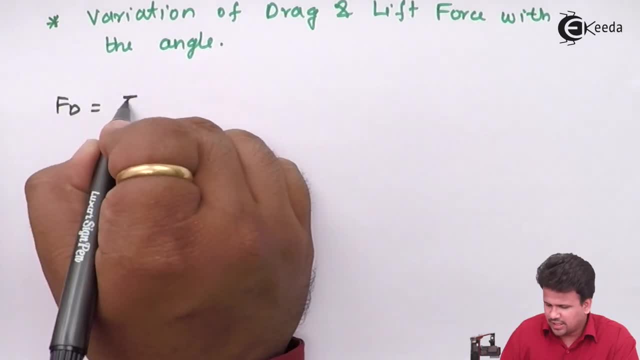 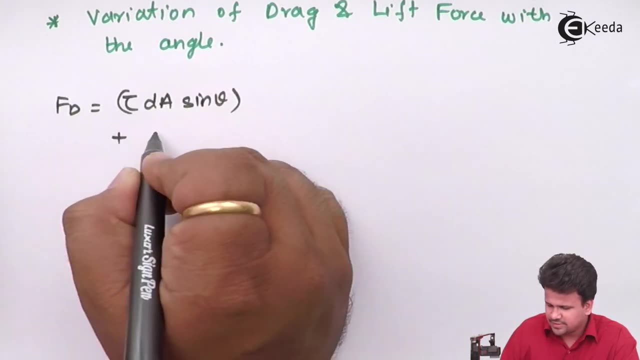 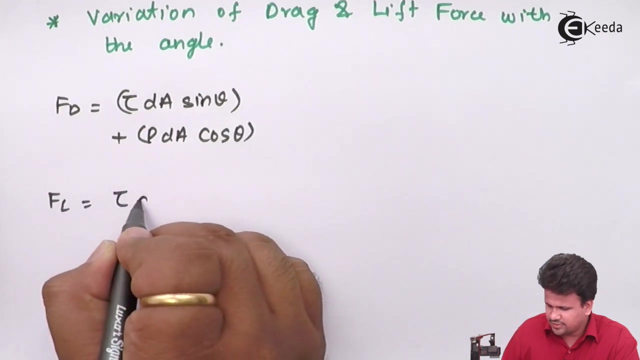 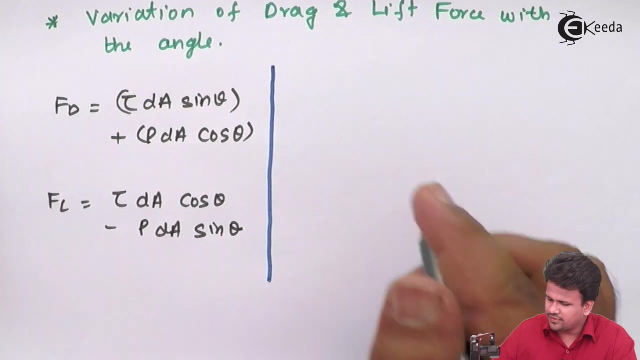 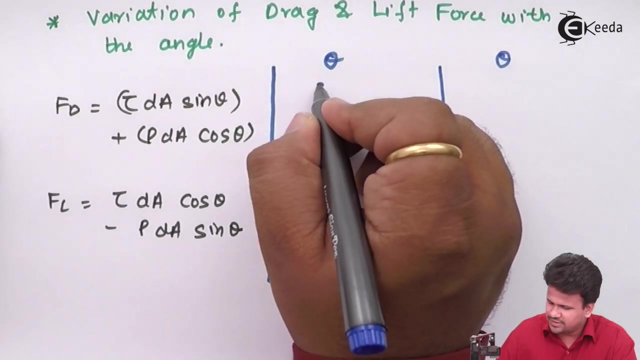 is equals to that is tau into da sine theta plus p into da cos of theta. Lift force is tau into da cos theta minus p into da sine theta. Now let us substitute over here the value of theta. So let us take theta is equals to 0. If theta is equals to 0,, 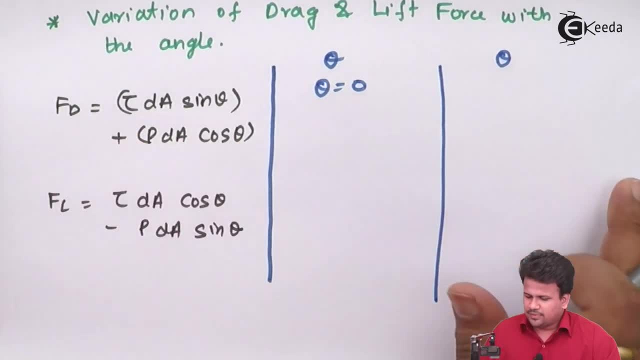 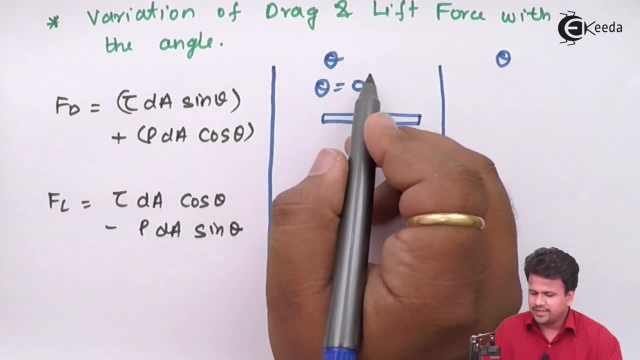 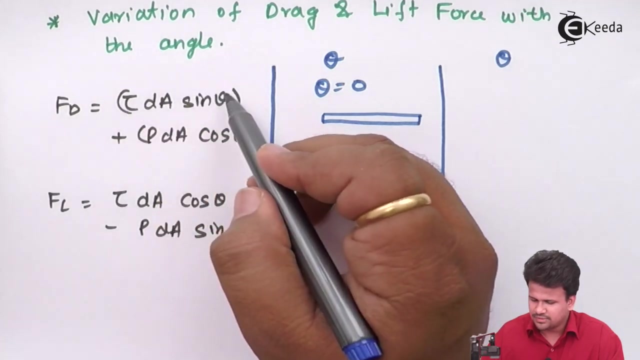 what happens is the entire body is actually horizontal, So there the angle is 0. So you can see over here, this part over here, which is the shear part, over here, That is the shear part, will tend to 0, will have the only pressure part, Similarly over here. 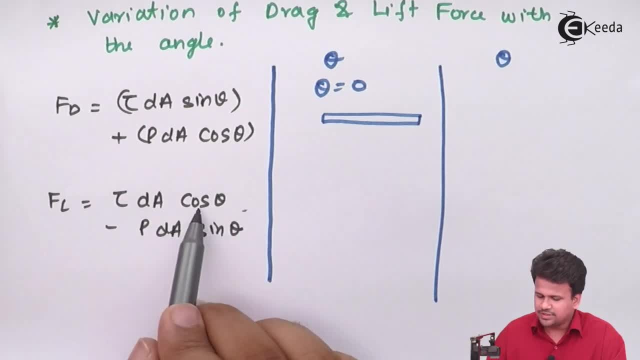 the pressure part will be 0. over here there will be only the shear part. Now, what do you understand by this? That is, the drag force will be larger when there will be the angle, which is 0. So drag force will be greater than the lift force. 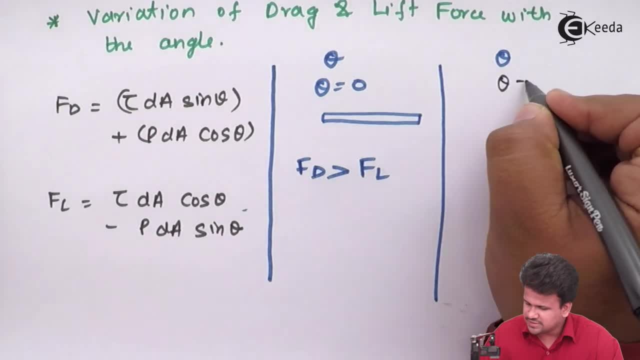 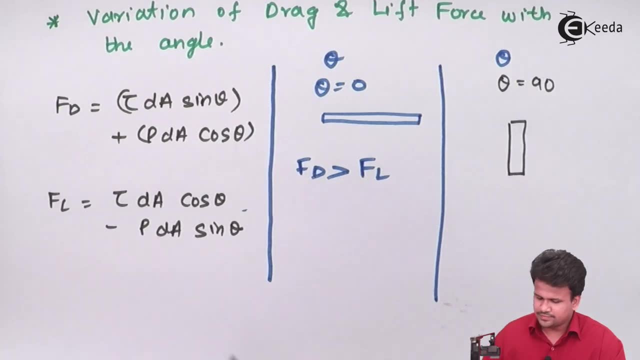 Now, if this angle is, theta is equals to 90 degree. what happens over here? So in this, in this part, the pressure part will be 0, whereas in this part the shear part will be 0. So 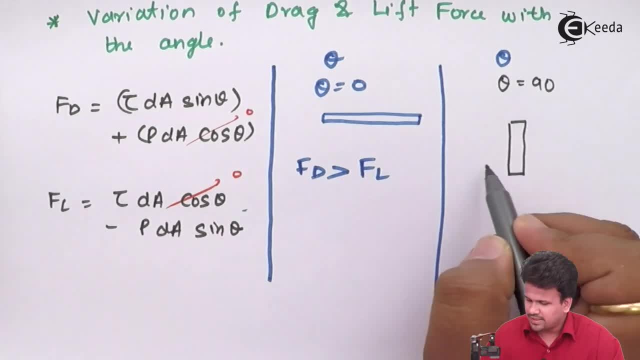 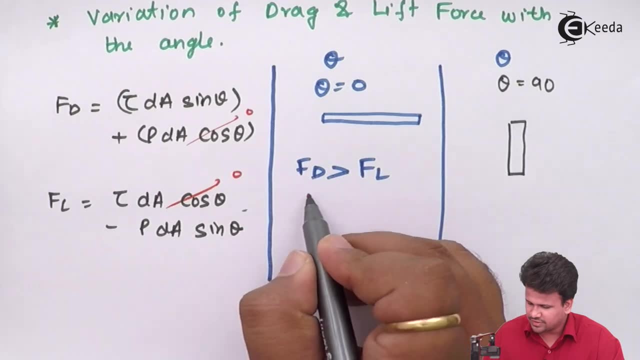 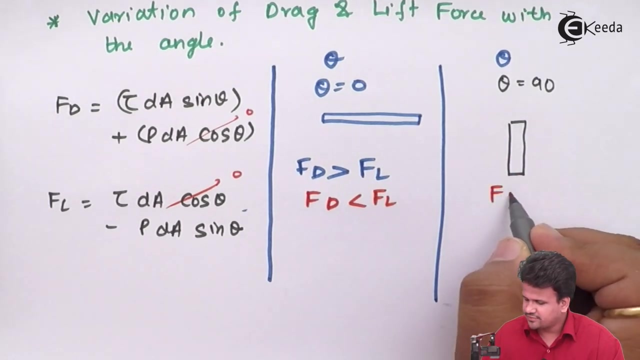 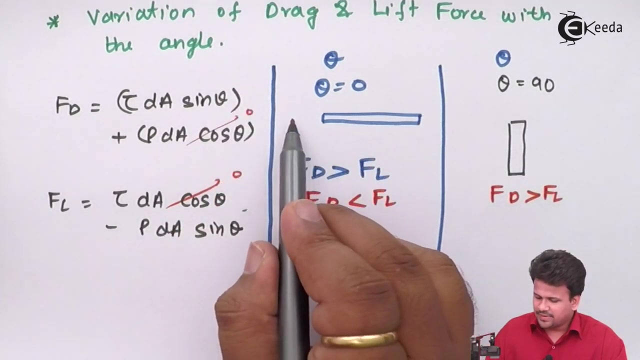 over here. what happens is when it is perpendicular, the drag force over here, rather the drag force over here in this, is less than, not greater than than the lift force. and it is perpendicular, drag force is greater than lift, for- just pardon my mistake- because over here the drag will be less, whereas the lift will be more. here, the drag will be more and the 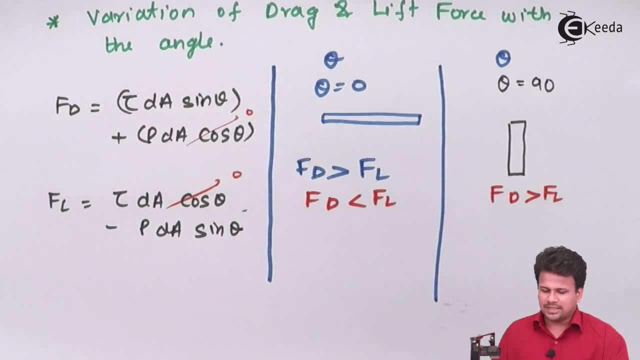 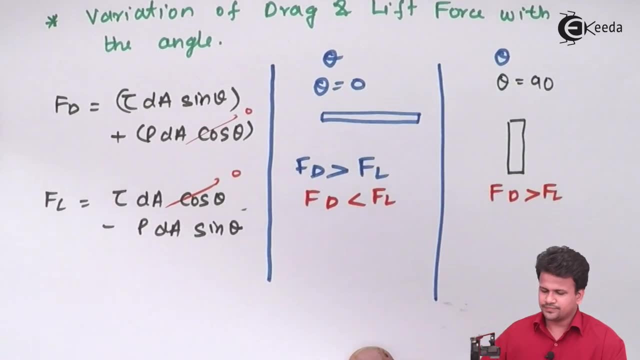 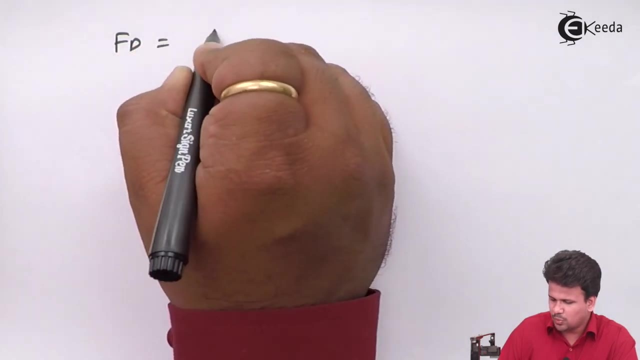 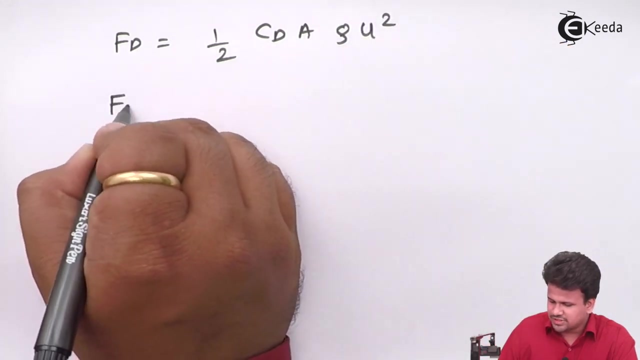 lift will be less, so that is depending upon the angle theta. now, final value of drag force according to coefficient of drag, can be given as fd is equals to one, half cd into a rho, into u square, and the lift force can be given as half into cl into a rho, into 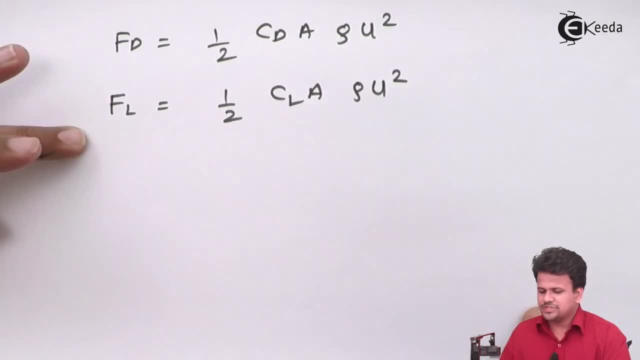 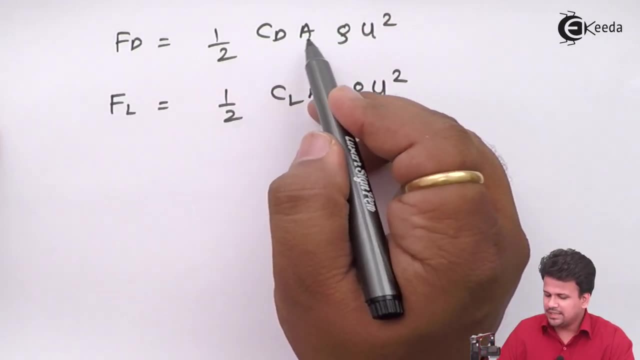 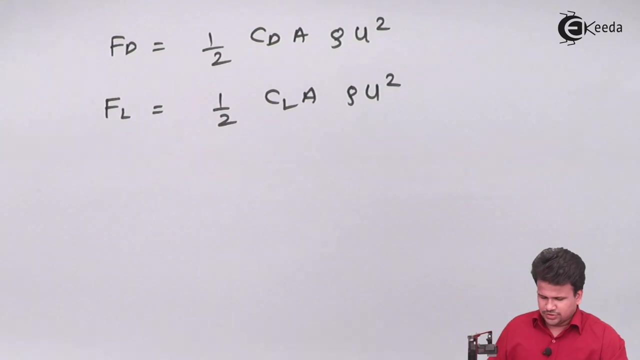 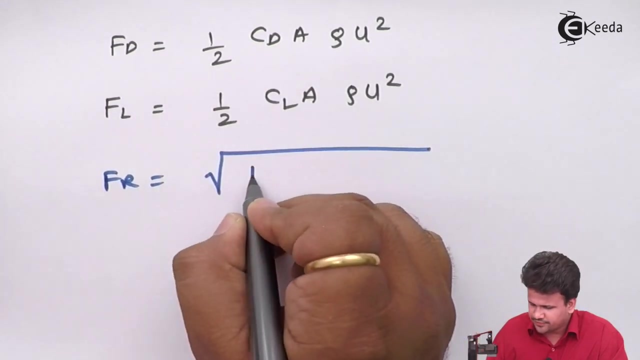 u square. so this is the drag force and lift force. when lift force and drag force are functions of velocity, it depends upon area velocity. coefficient of drag and coefficient of lift remains constant. so that remains constant and the total force will be vector sum of f d square plus f l square. 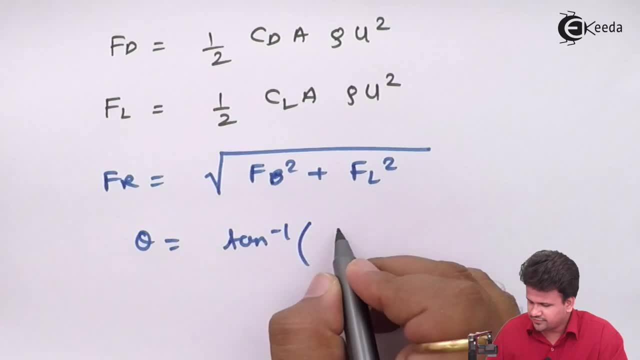 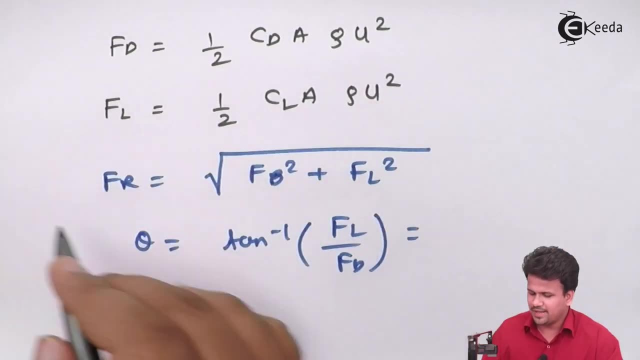 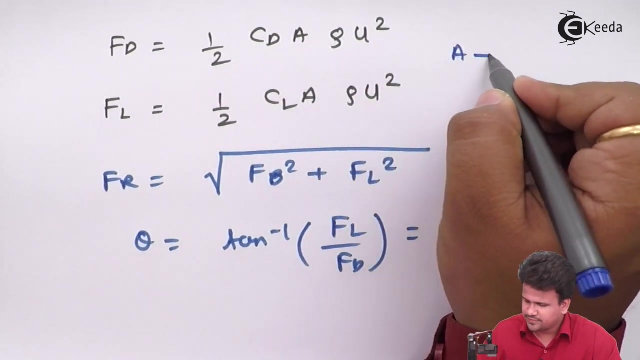 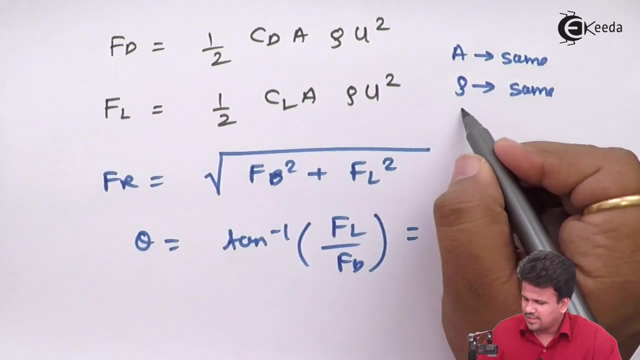 theta will be equals to tan inverse of lift force by drag force. if the velocity is same, all the parameters of same, then it will be equal to tan inverse of: if the area is same, a is same, density of air is same for both of them, of course the velocity will be also same. then it will be ratio of 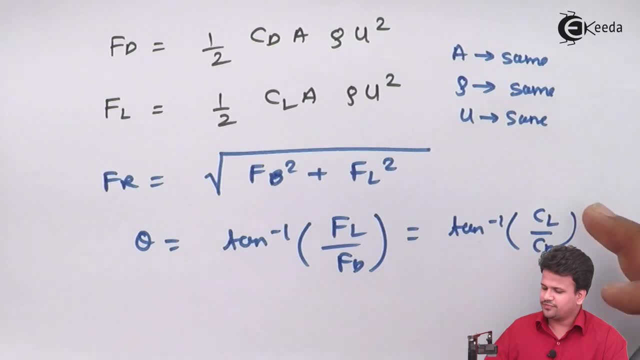 the drag force and lift force and this is equal to the drag force over cd, that is, the drag coefficient of lift force to the coefficient of drag force. so i hope you have understood how we have calculated the drag force and lift force and what is actually a drag force and